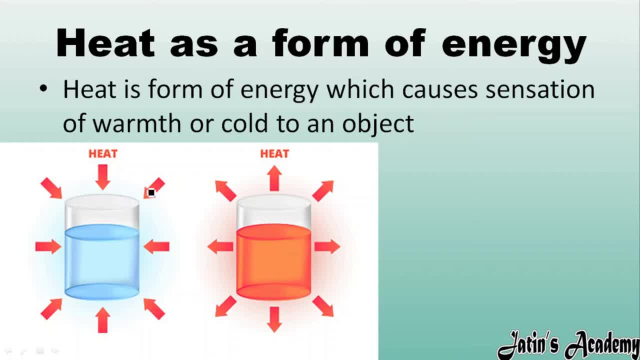 is coming inside the water from the environment. Whenever too much heat is coming inside the water means this water starts to heaten up. Ok, And whenever from the water heat is going out of the water. and when heat is going out of the water. 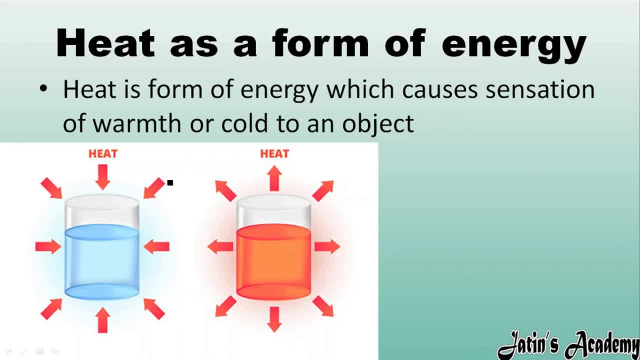 Then you can say: this water is becoming cool, Ok. Whenever heat is going to any object, that object is becoming warm. Whenever heat is coming out of any object, means object is becoming cold. Ok, So in accordance with the heat. actually, heat is a form of energy which enables us. 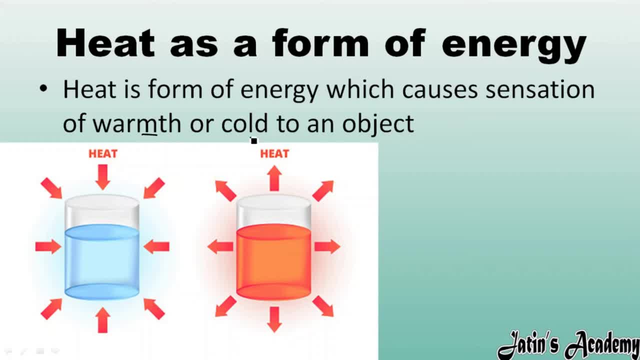 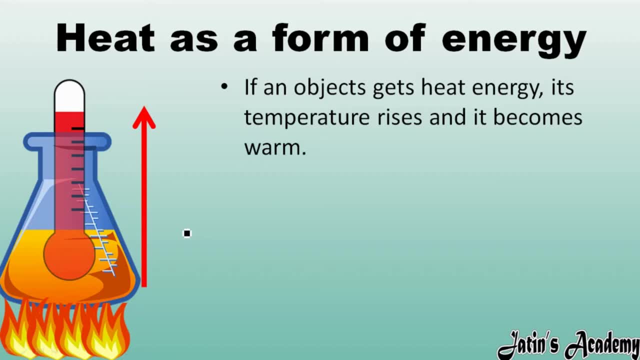 to sense that which object is warm and which object is cold. Fine, So next we are having in relates to temperature, how heat work. Actually, whenever we are given too much heat to any object, Giving heat to object means the temperature of that object rises, Whenever we are giving. 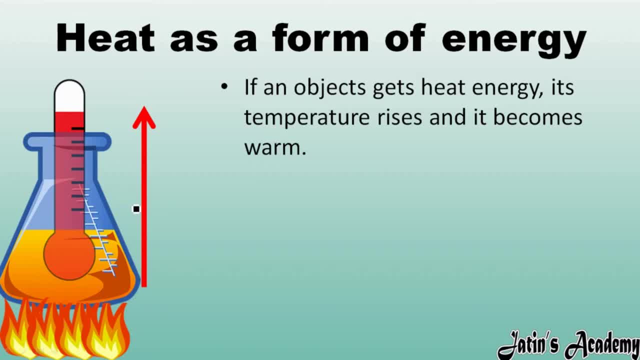 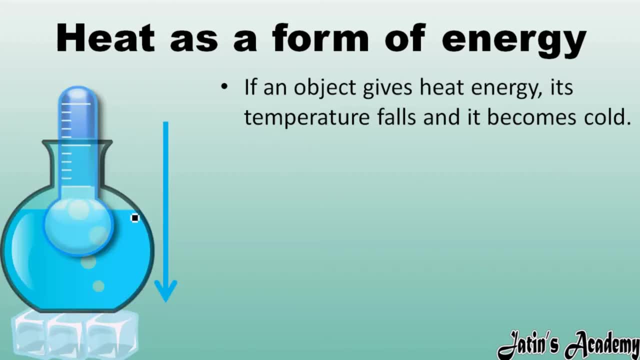 heat to any or heat energy to any object, The temperature of that object rises and this object will become warm. And similar manner if we are giving heat energy out from that body. If heat energy is coming out from that body, you can say the temperature of that liquid. 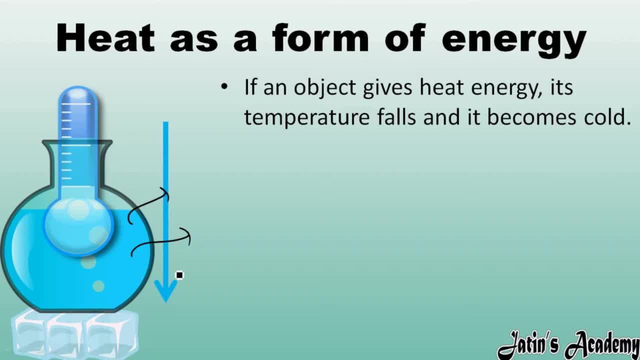 or that object falls and that liquid will become cold. So two things are there: either temperature can fall, or either temperature can rise Whenever the temperature of that object is coming out from that body. you can say the temperature of that liquid or that object can rise Whenever we are giving too much amount of heat to any body. in that case, 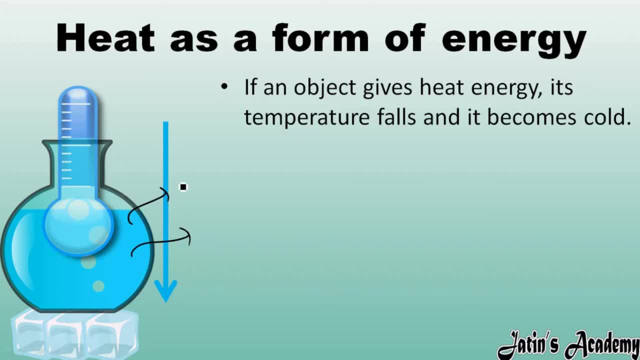 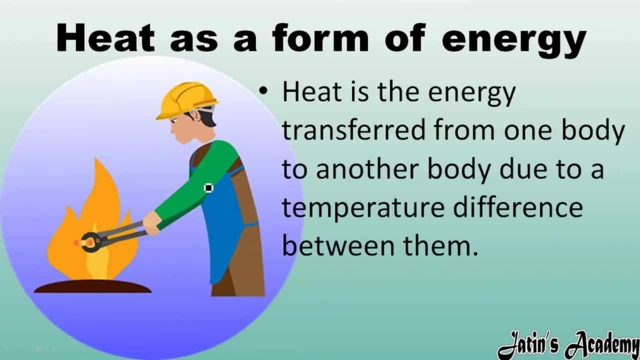 temperature increases and whenever we are taking heat out from any body, in that case temperature reduces. So next we are having heat is the energy transferred from one body to the another body due to temperature difference Whenever we are taking any object and we want to heaten up this object. How we will heaten up? First of all, we will tong and we will. 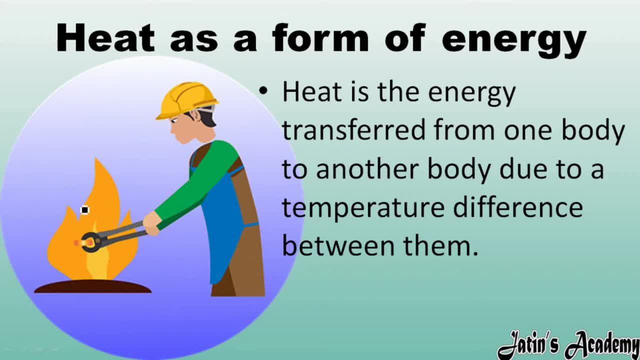 put that object into a fire. Ok, Till the point when the temperature between this fire and this object will become same. till that point this object will heaten up, Ok, So what do you mean by in this temperature difference? Temperature difference means whenever two. 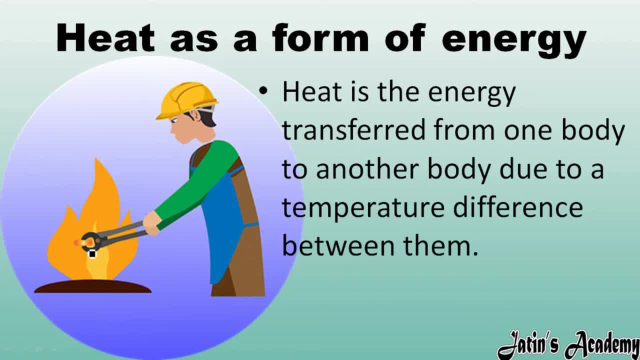 objects are there of different temperature. Firstly, this object is having low temperature and fire is having high temperature. Ok, And when we are combining these two different temperature, heat is going to move from higher temperature to the lower temperature and till that point heat will move till both. the temperature of the object is going to same, Ok, So this's 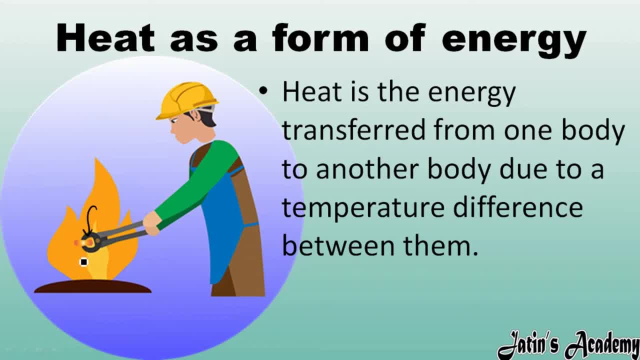 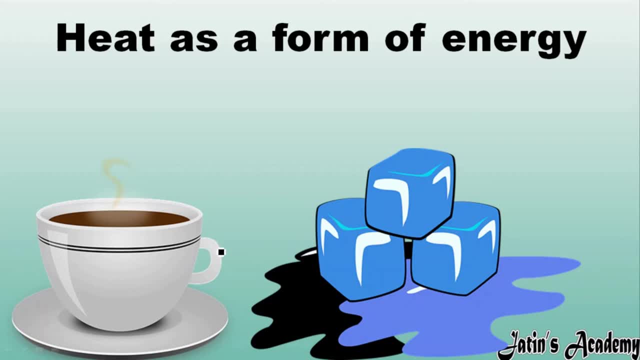 way you can learn that heat can always move from higher temperature to the lower temperature. So here we are having the example that how heat move from higher temperature to the lower temperature. For example, in this cup we are having hot tea. Hot tea means temperature. 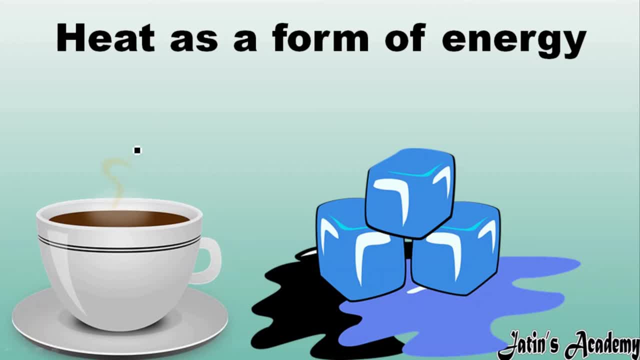 of this tea is very much high, but if we will do the comparison between the tea and the environment, in the environment temperature is less as compared to tea, So here heat will move, from which? Heat will move from higher temperature to that of lower temperature. 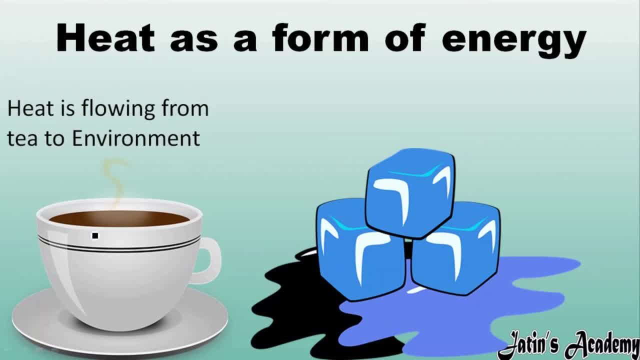 Similarly, the heat flow from tea to the environment, or you can say higher temperature to the lower temperature, But in the case of ice cubes, actually ice cubes are having low temperature. In ice cube temperature is low, but the environment temperature is high as compared to ice cubes. 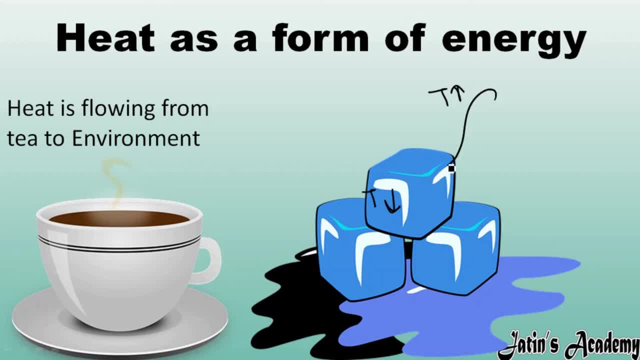 So this temperature or this heat will move from higher temperature to the lower temperature. When heat move from higher temperature to lower temperature, ice cubes starts to melt. In a case of ice, heat is flowing from environment to the ice Clear Or from the higher temperature. 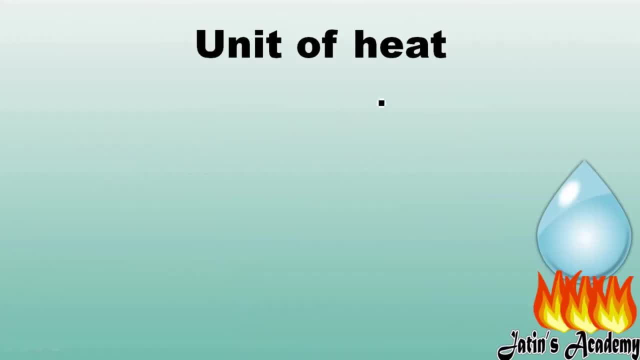 to the lower temperature. next topic: we are having unit of heat. as we know, each and every physical quantities are having its own unit. like they are having SI unit, they are having CGS unit. in a similar manner, heat is also having some its SI unit as well as its CGS unit. so SI unit of heat. 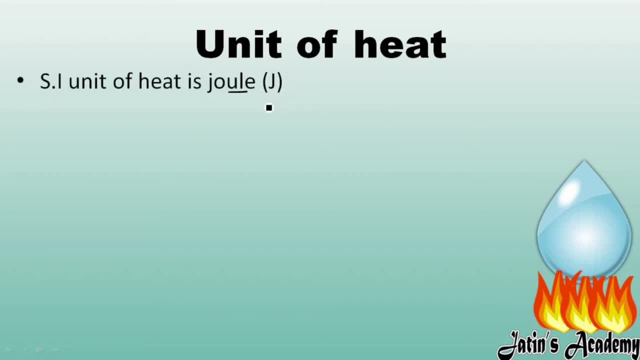 is joule, you can represent it by capital J and CGS. unit of heat is calorie. okay, these two units you have to learn as a SI and CGS unit of heat. now we are going to see the relation between SI and CGS unit of heat. so here we are having the relation. as you know, calorie is the CGS unit. 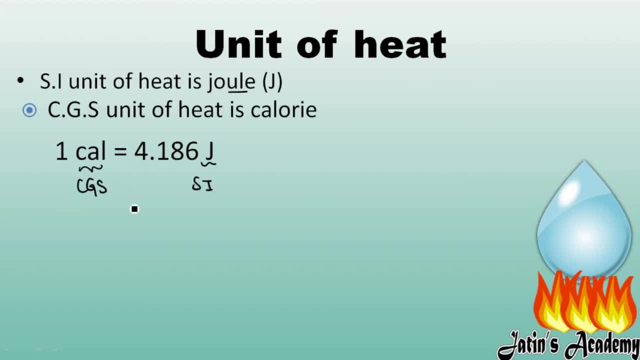 and joule is the SI unit. so here is the relation between CGS and SI unit of heat. that is, one calorie is equals to 4.186 joule. or you can also learn like this: one calorie is approximately equals to 4.2 joule instead of 186. or you can round off, you can write 4.2 joule. next we are having definition. 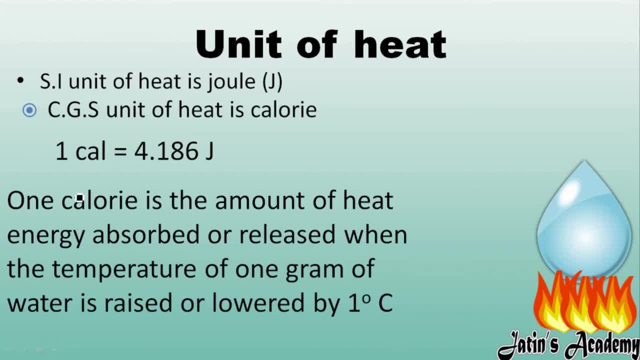 of one calorie. so in which case you will say you can write 4.2 joule, so in which case you will say that, yes, this heat is having one calorie of unit. so actually here you have to take one gram of water, and what we have to do here, actually, if you want to increase the temperature by one degree Celsius. 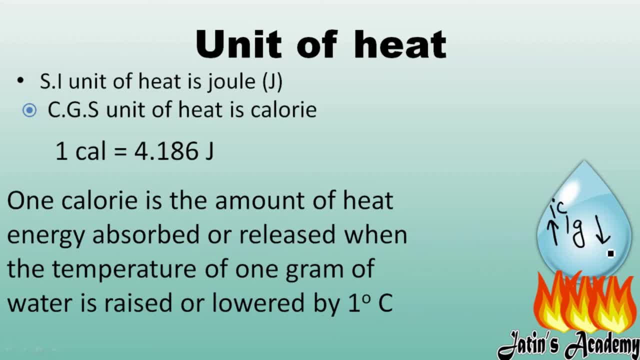 of this one gram water, or you want to decrease the temperature of this one gram of water by one degree Celsius. in both the cases, you have to either give the heat energy to this one gram or you have to take the heat energy out from the one gram of water and this amount of heat energy. 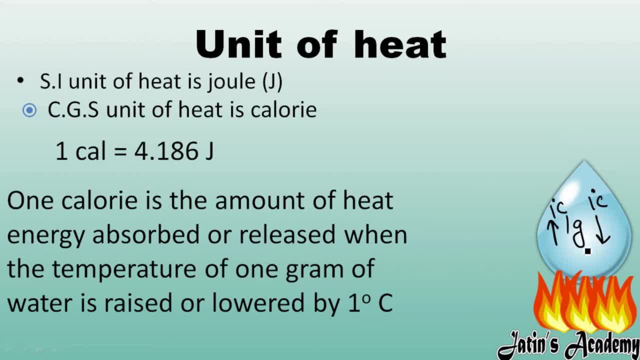 absorbed or released. when the temperature of one gram of water is raised or lowered by one degree Celsius is known as one calorie. clear the definition of one calorie. so here we are having bigger unit. as we know, calorie and joule are the CGS and SI unit of heat and kilo calorie is the bigger unit of heat. if you want to measure the 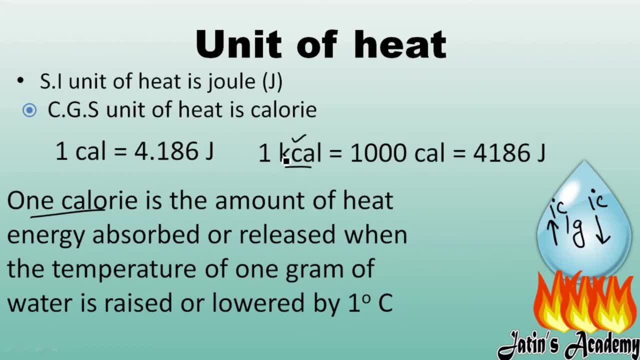 heat in the bigger unit, then we will use kilo calorie. so, as we know, in one kilo calorie, kilo means thousand. so one kilo calorie means 1000 calorie. and if you want to write in the form of joule, so one kilo calorie is equals to four kilo calories. so one kilo calorie is equal to four. 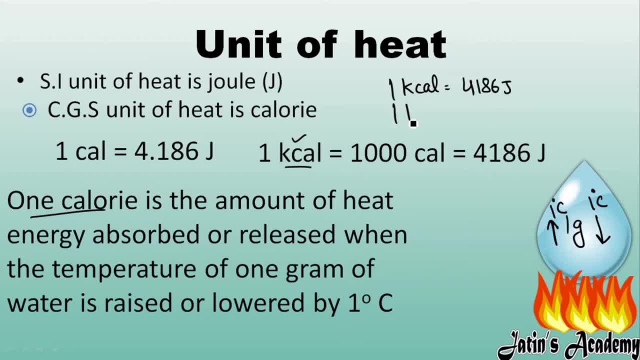 186 joule. or you can write like this also: 1 kilocalorie is equals to 4200 joule. these relation you have to learn because these are very important from exam point of view. clear. next we are having the topic effects of heat. so what? what are the effects of heat whenever we 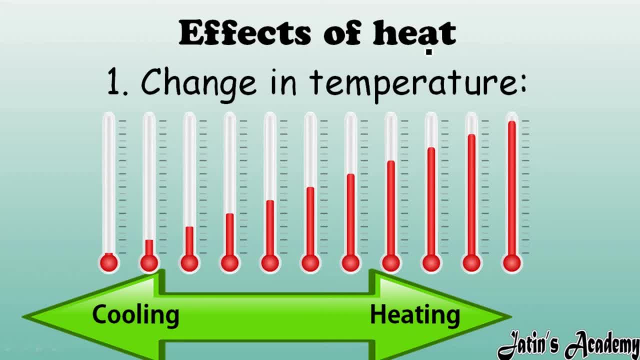 are giving heat to any body, whatsoever changes we are going to see in that body. so very first change we are having change in temperature whenever we are giving temperature or whenever we are giving heat to any body. heat to anybody means that body is changing its temperature. while taking heat its temperature increases. and while taking heat out from anybody, or you can see- 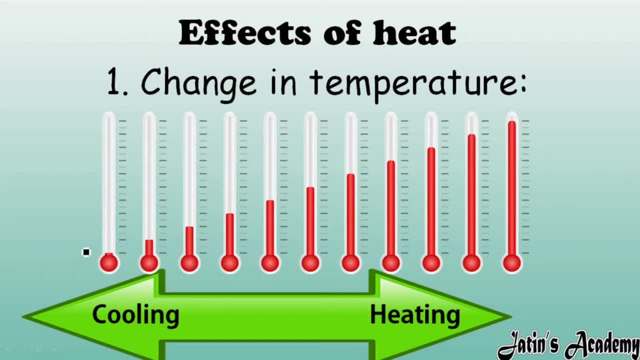 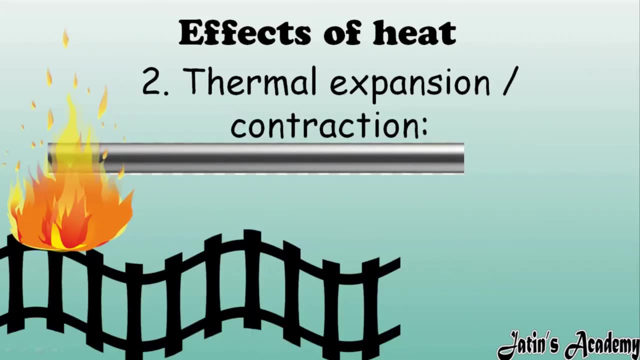 while cooling anybody, temperature of that body is going to reduces. so whenever we are heating to anybody, heating increases, temperature increases. whenever we are lowering the temperature or we are cooling something, heat low. so here temperature is also low, clear. next we are having second effect of heat, that is, thermal expansion and contraction. so actually whenever we are giving heat to any body, 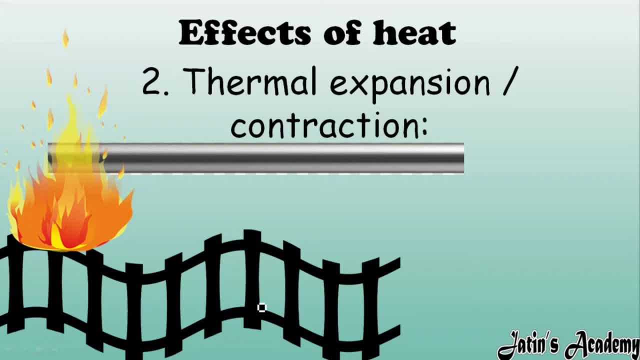 that body is going to expand by its length, breadth as well as height, wise, okay. so when, for example, here i'm going to give the heat to this body, this body is going to increase its length means it is doing thermal expansion. and in a similar manner, if i am taking heat out from any body or we are, 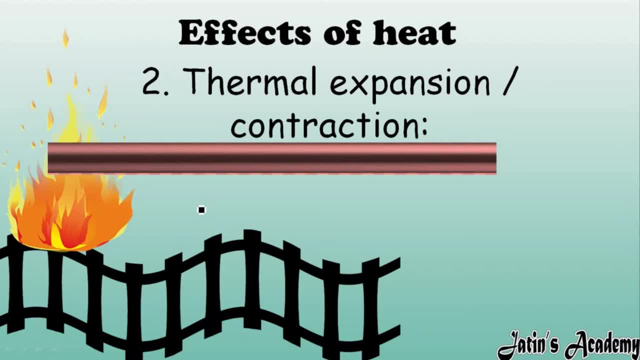 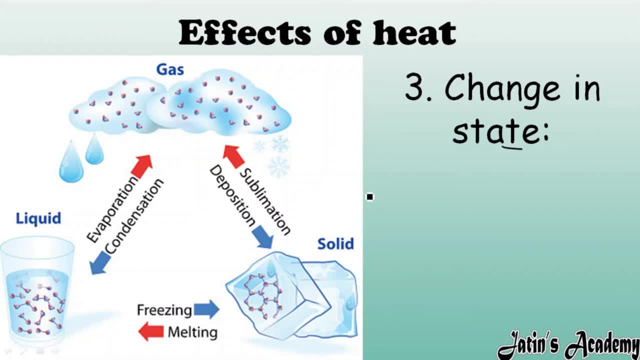 cooling any body. in a case of cooling there is a thermal contraction means that body is going to contract. okay. next effect of heat: we are having change in state. so whenever, for example, we are having any solid and we are giving heat to this solid, so obviously this solid will converts into 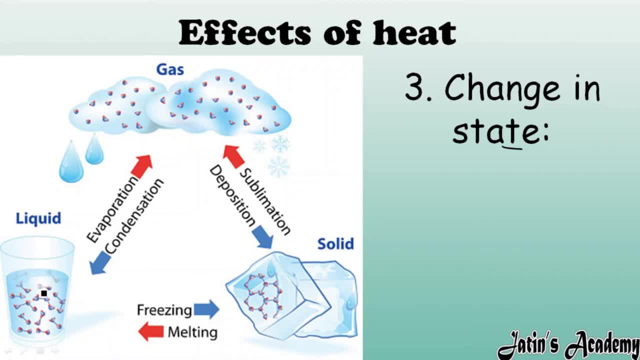 a liquid and when we are further giving heat to this liquid, this liquid will convert into gaseous state. means by giving the heat we can change solid to liquid or you can change liquid to gas. but yes, in the second case also, if we are taking heat out of any body, means if i am cooling this liquid. 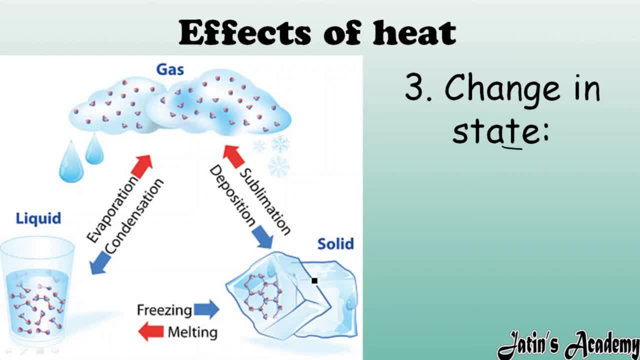 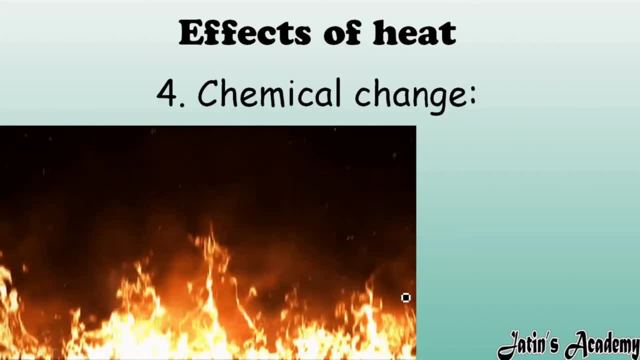 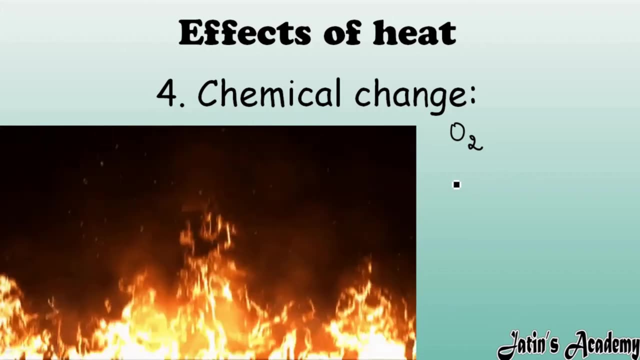 this cooling of liquid will converts into solid state means we are changing the state by the effect of heat. next effect of heat: we are having chemical change. chemical change means what? whenever we are giving heat to any object in the presence of oxygen, burning is there. whenever we are burning to any substance, burning will always. 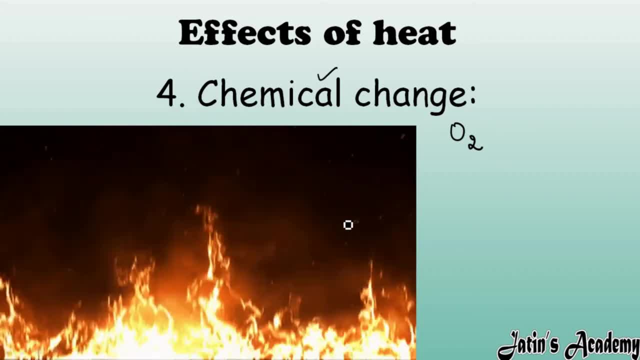 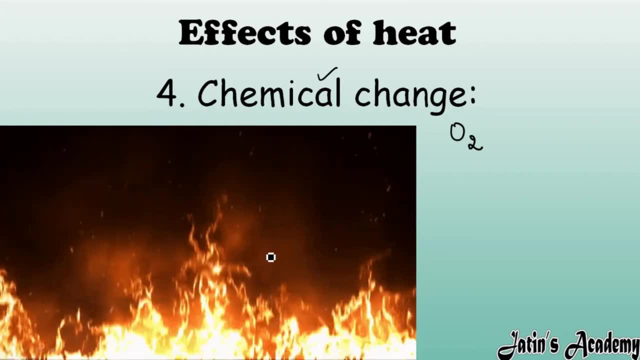 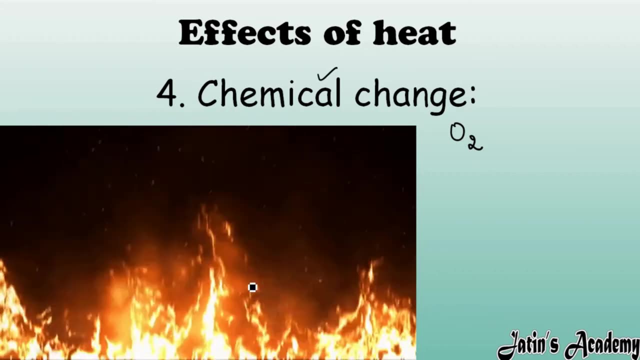 cause a chemical change. chemical change means the chemical properties of that material is going to change, means after changing its chemical properties. for example here, paper is there whenever we are burning the paper. firstly, paper is having its different properties, but while burning or while giving the heat, this properties of the paper almost changes and it converts into 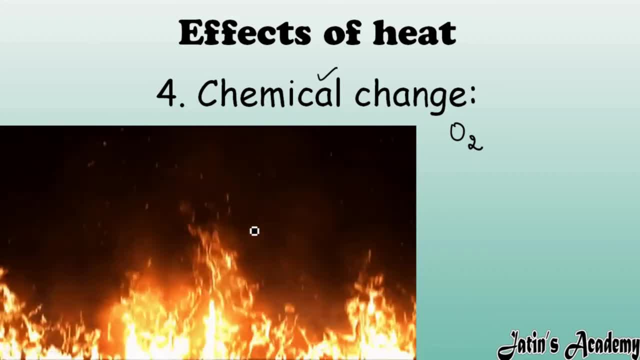 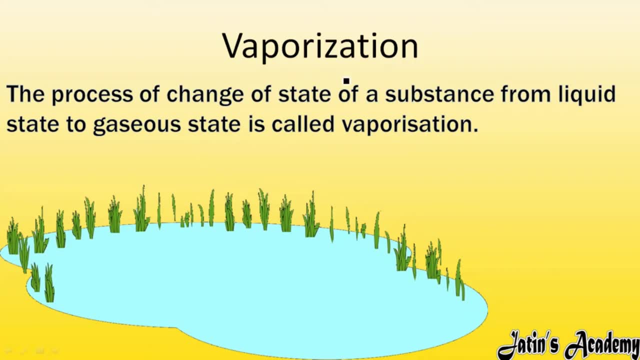 for example, carbon dioxide, light and ash. okay, so there is a chemical change whenever we are giving heat to anybody. so next topic: we are having vaporization. so what do you mean by vaporization? see carefully. actually, vaporization is a process in which there is a change of state from the 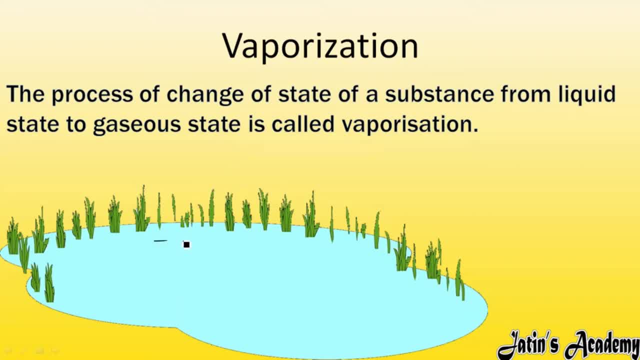 liquid state to the gaseous state. whenever liquid changes to the gaseous state of matter in that process, or in that case, you will say that it is a vaporization process. okay, so this vaporization process can takes place by two methods, and what are that? 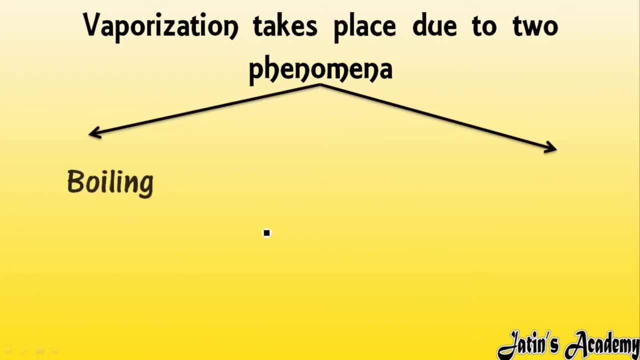 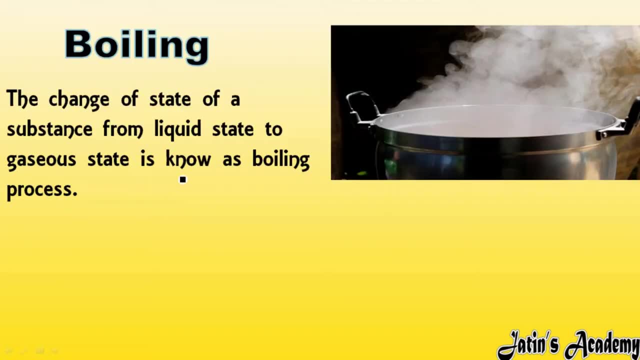 two methods, see carefully. first method: we are having boiling and second, we are having evaporation. so one by one in this chapter we will discuss about what is boiling and what is evaporation. so first method of vaporization: we are having boiling. so what do you mean by boiling? see 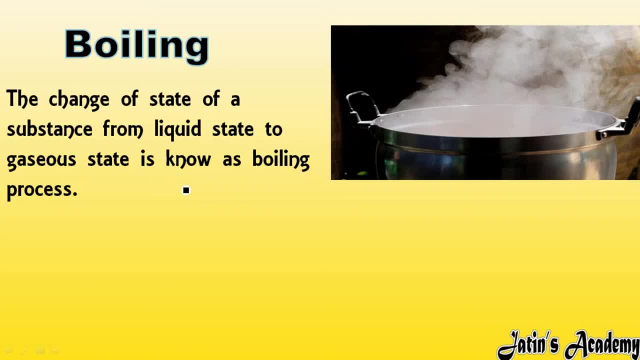 carefully. actually, in a boiling, there is a change of state of liquid state to the gaseous state. okay, this is known as boiling process, but boiling takes place only at a fixed temperature or a fixed point. that fixed point is known as, or that fixed temperature is known as, boiling point- whatsoever. 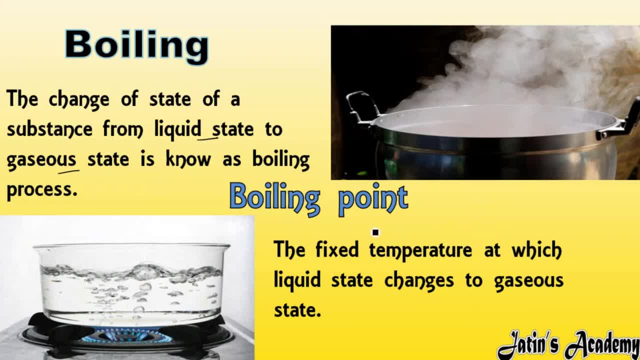 liquid we are taking in order to convert it into the gaseous form. that liquid will only converts into the gaseous state only at a fixed temperature and that fixed temperature is known as boiling point of that liquid. for example, if i am taking about the liquid that is a water, if i am talking, 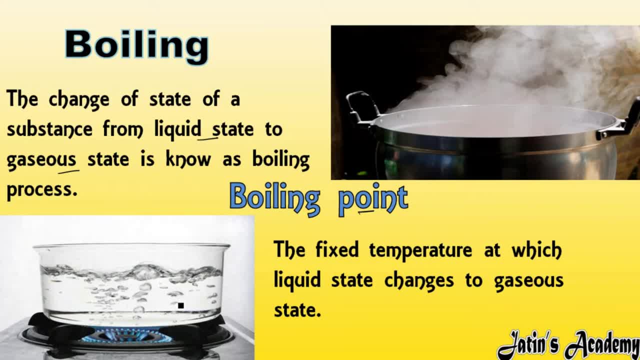 about the liquid, that is, a water at a fixed temperature. that temperature is known as boiling point. okay, and this boiling point is always 100 degree celsius. if you are taking different liquid, different liquid is having its different boiling point. so next question: is there that how boiling process occurs means how 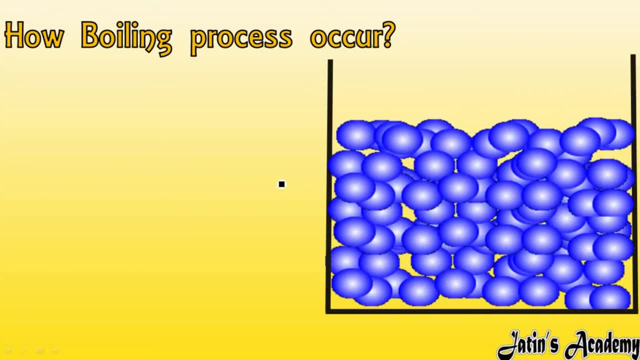 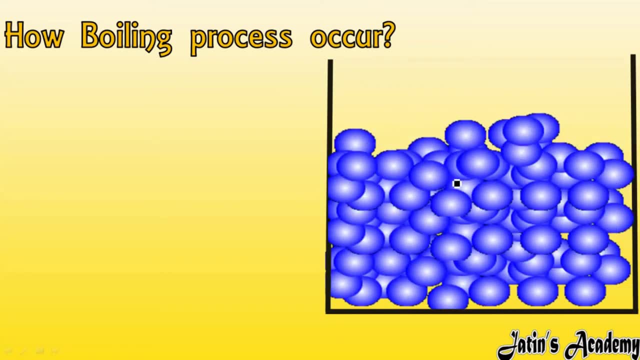 from the molecular theory boiling occur, how the liquid changes into the gaseous form. so see carefully, for example, here i am having a container. in this container liquid molecules are there. so the liquid molecules are randomly moving here and there. okay, but whenever i am giving the heat in, 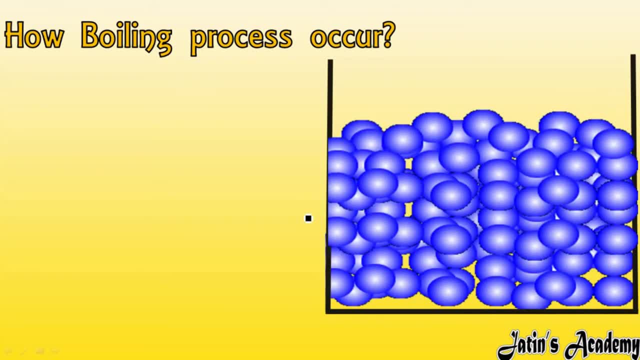 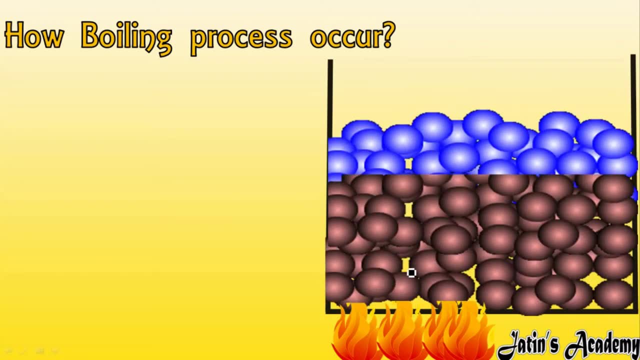 the liquid state of matter to the gaseous state of matter by giving the heat to this liquid whatsoever. the nearby particles are there. that particles will gain the energy from heat. they are going to heaten up and these particles then transfer the energy to next particles. next. 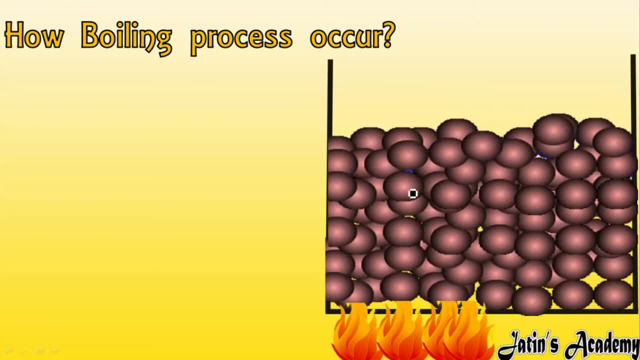 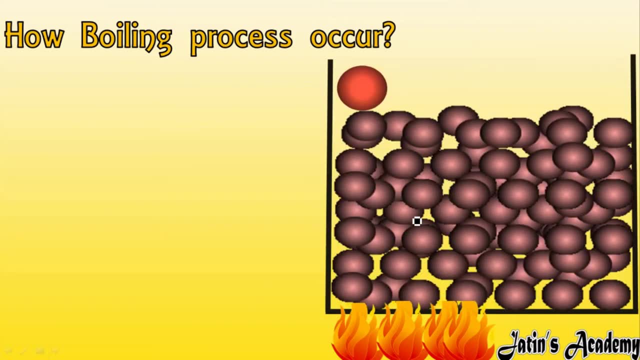 particles are also going to heat up by this, full-fledged particles whatsoever present in the liquid that is going to heaten up and due to this energy, taking from the heat what they are doing, whatsoever force of attraction between the particles, that force of attraction going to become. 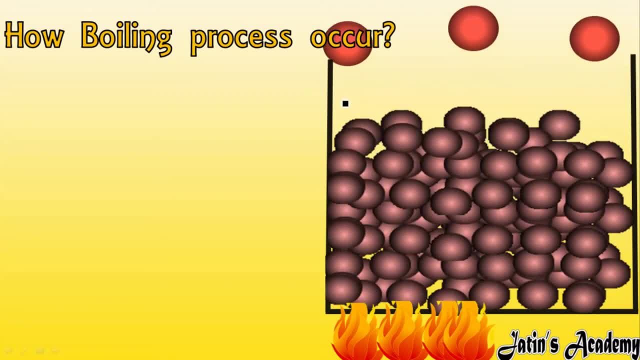 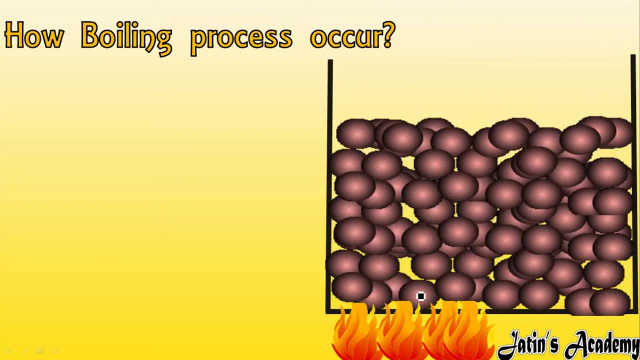 able to move away from the liquid particles means, first of all, here, free surface is there from which liquid particles cannot move away. but now, by gaining the energy from the fire or by the heat, what they are doing, they are just minimizing the energy between the molecules by minimizing the 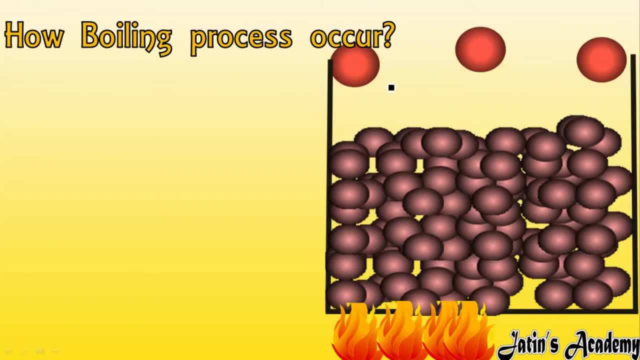 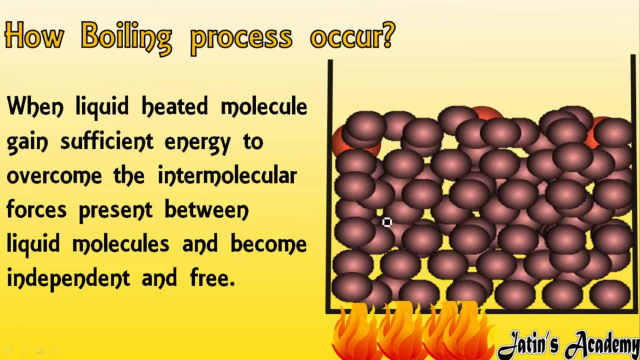 energy between the molecule. they are just converting into the gaseous form, so the liquid changes into the gaseous state. okay, so here we are having the full-fledged explanation for the how boiling process occurs, actually whenever we are having the liquid molecules and when we are. 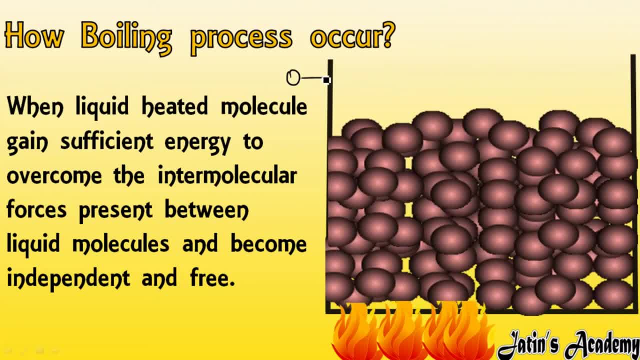 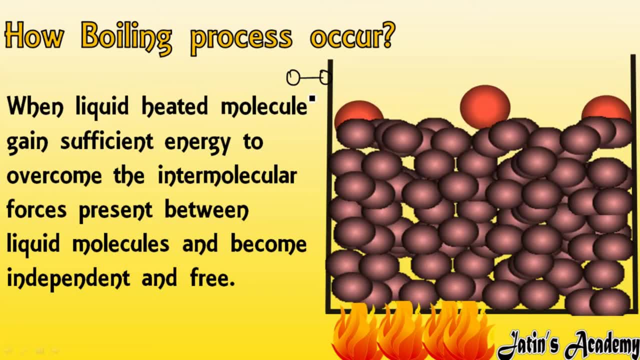 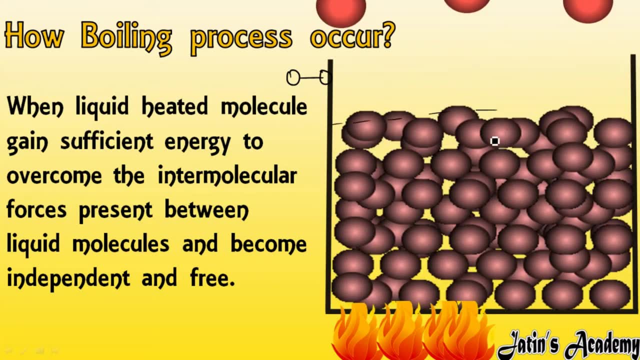 having the liquid molecules, they don't gain the sufficient energy in order to overcome the force of attraction between them whatsoever. force of attraction is there. by taking the heat, these force of attraction are going to weaken up. and by making this force of attraction, liquid particles are now able to move away from their free surface. means this free surface now they are. 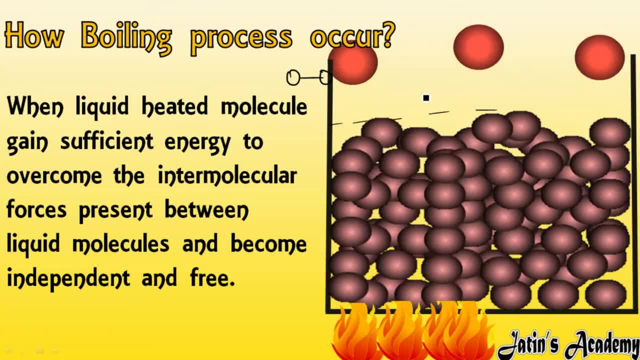 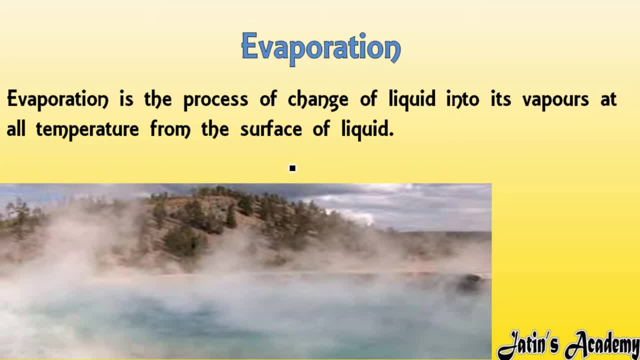 able to move away. by converting into the gaseous form, they can move into the atmosphere. next method of vaporization: we are having evaporation. so what do you mean by evaporation? see carefully: in evaporation, also like a boiling, there is a change of liquid state of suffering, which means, if we are 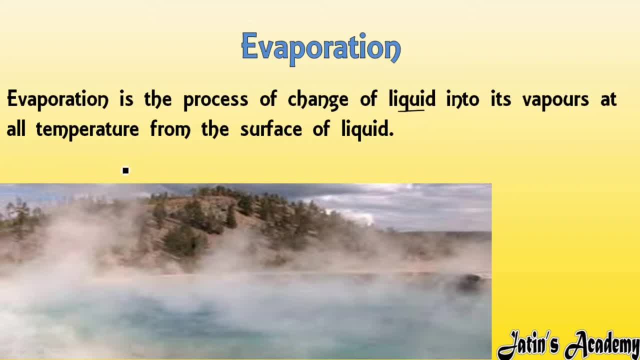 changing the vaporization. it is going to change its form, closing the vaporization of the liquid, and we are going to be able to have vaporization, which means water is being released by vaporization then of matter into the vapor state, or you can see gaseous state of matter, but here, like the boiling, 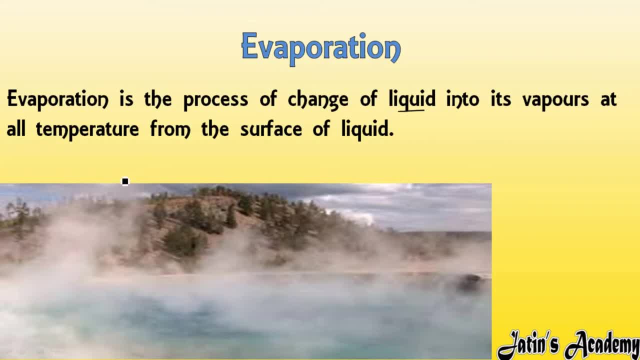 it is no need of the boiling point in this evaporation. evaporation can takes place at all temperature. at all temperature, yes, but below the boiling point means here: if the temperature is below the boiling point, in that case only evaporation occurs, means the liquid changes into. 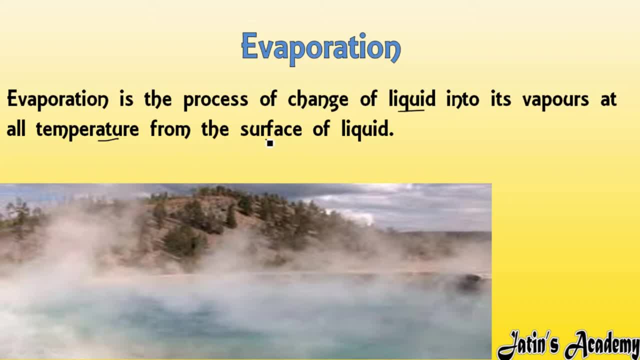 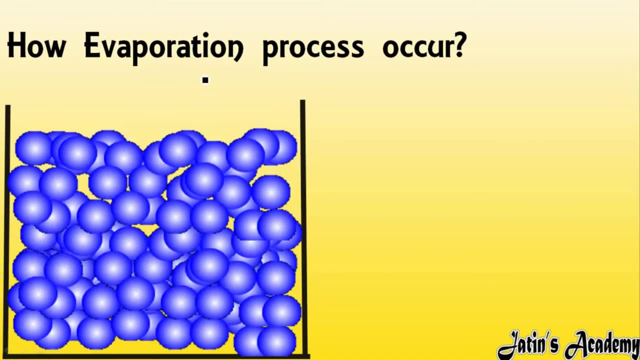 the gaseous form, but evaporation occurs only at the surface of the liquid. this i will explain you in the next slide. so now we will see how evaporation process occur means how the change of liquid state of matter is there, into the vapor state or into the gaseous state, how evaporation 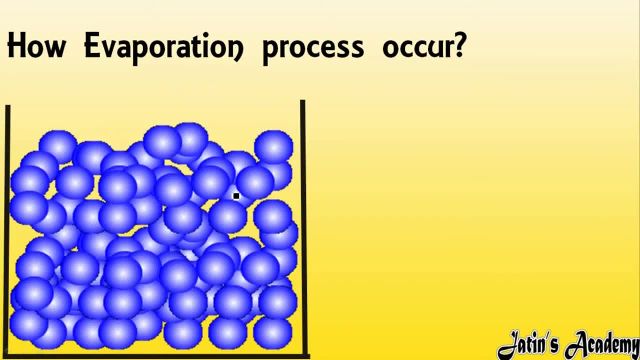 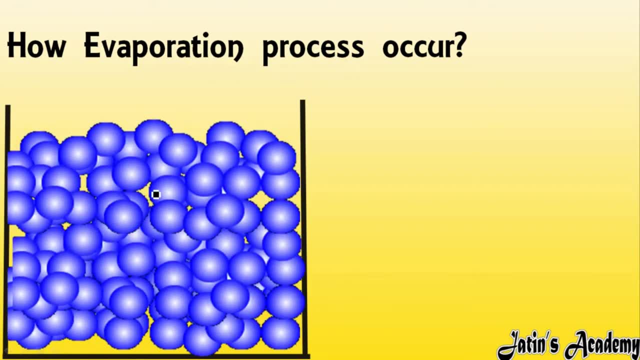 occurs. see carefully. for example, here also i am having a beaker in the beaker. liquid particles are there now. the molecules of the liquid are randomly moving here and there. but these molecules are having this much amount of force of attraction that they cannot leave their free surface means. 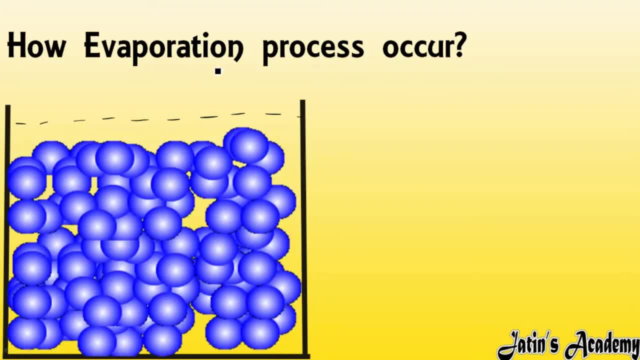 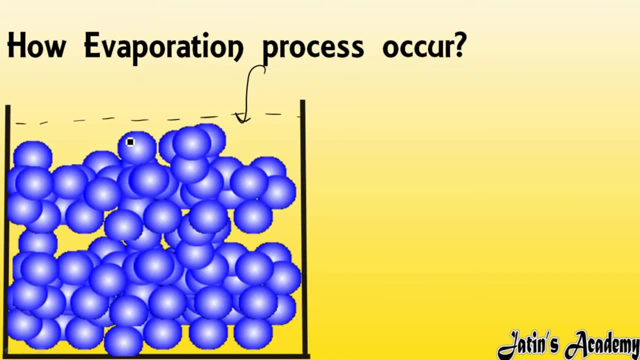 liquid cannot move up from their free surface. they cannot move away from each other. okay, but whenever there is a gain of energy from the surrounding, either from the surrounding or the upper layer of the molecules, will take up the heat from the lower layers of the molecule or from the lower molecules. 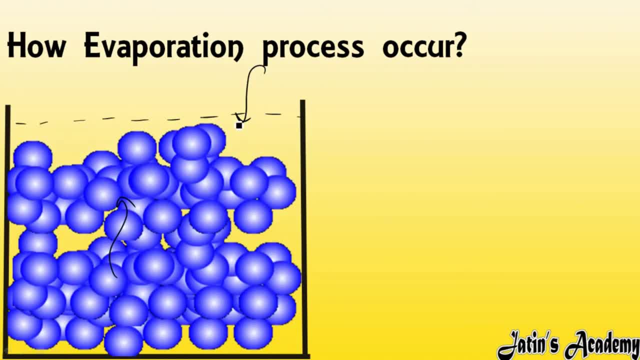 what they are doing. the upper layer: firstly, take the heat, either from the outside, either from the lower particles. these particles or these molecules are going to take the heat and by gaining the heat, whatsoever energy is there or the force of attraction is there between them. that force of attraction is become too much weak that they can overcome this. 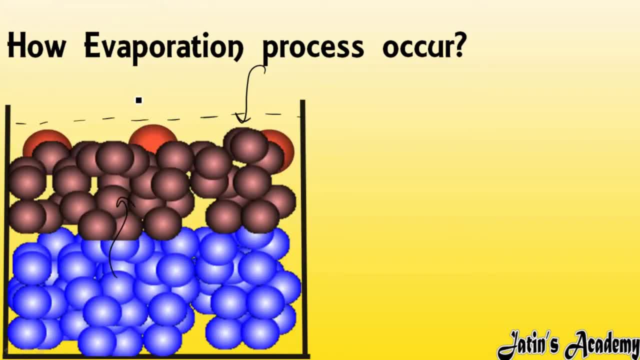 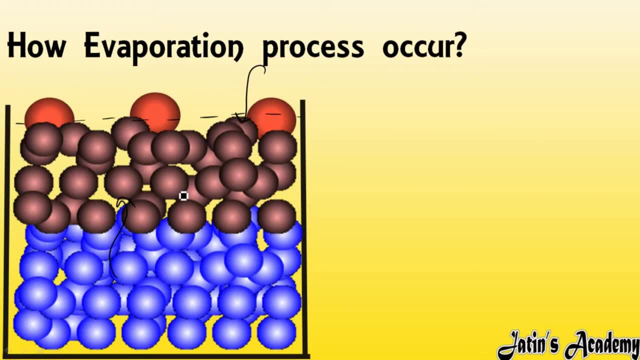 free boundary or free surface. they can move away from it and the liquid particles or liquid molecules now are able to convert into the gaseous form. okay means in evaporation, not full-fledged, is liquid going to heat and up? only the upper surface is going to. 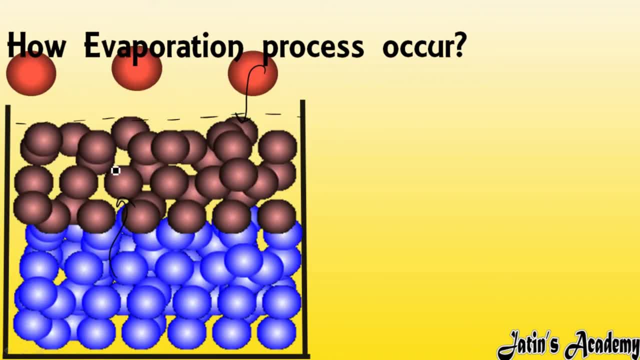 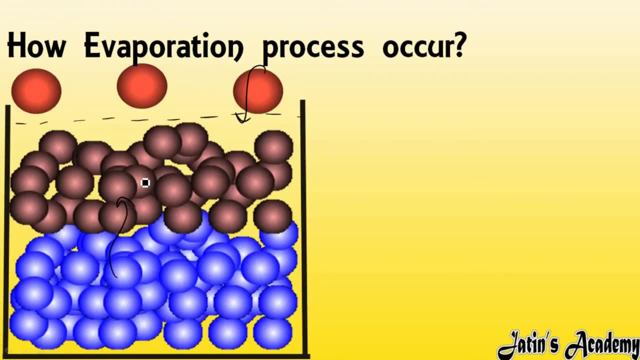 take up the heat or from the lower surface, it is going to take up the heat. by taking the heat, there is a weakening of the force of attraction between the particles. due to weakening of the force of attraction between the particles, now the molecules are able to convert from the liquid. 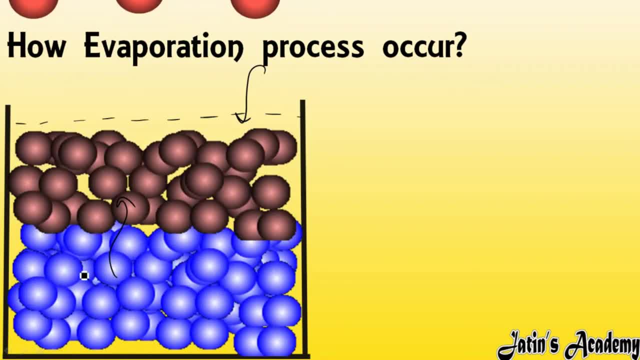 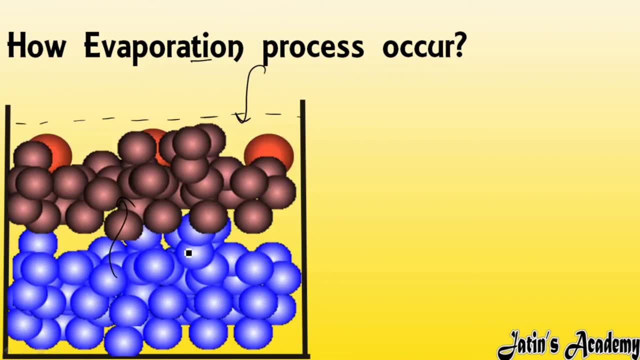 state to the gaseous state. okay, by losing the heat, these molecules will gain up the cooling effect. that is why, whenever there is a evaporation process behind the evaporation process means whenever there is a change of liquid to the gaseous state of matter, behind it there is always 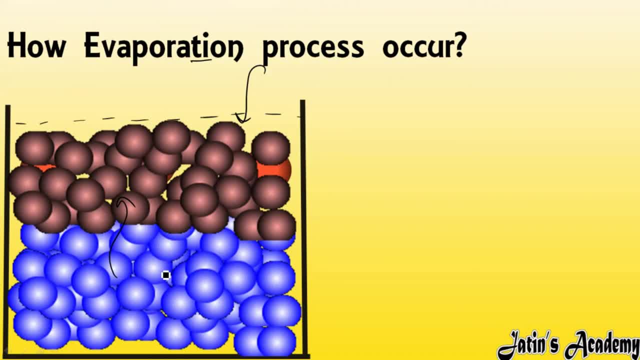 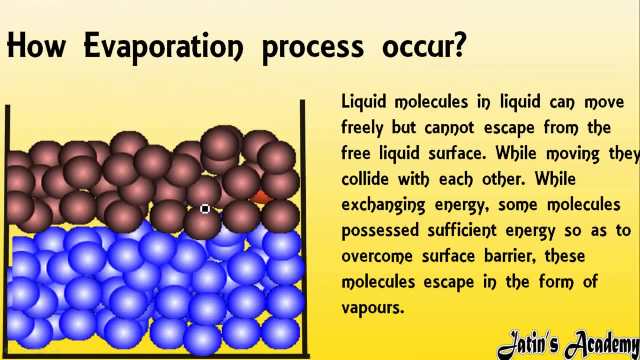 a cooling effect. okay, after evaporation, there is always a cooling effect seen during the evaporation. so here we are having the theory that how evaporation process occurs in this liquid molecules are free to move. okay, these, but these molecules are having this much force of attraction. 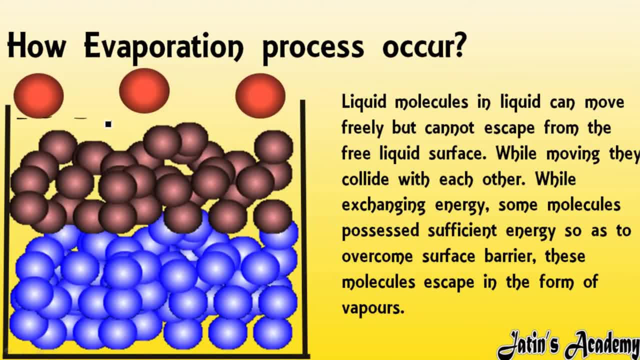 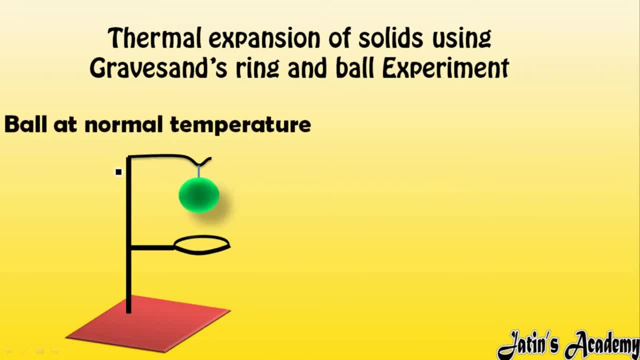 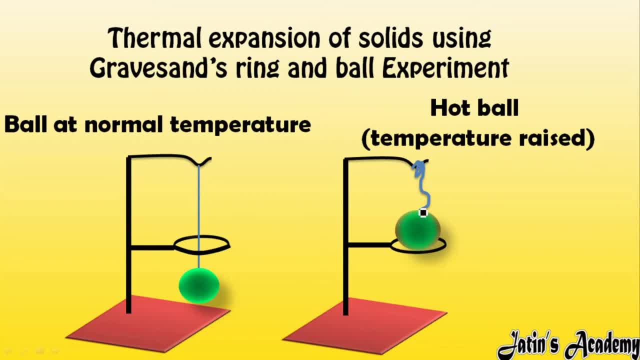 size of the solid. due to expansion of size of the solid now this ball is not able to move from this ring. that is why it shows us that whenever we are heating any solid, there is expansion in a solid. so this grave sense ring and experiment ball is there in order to show the thermal expansion in 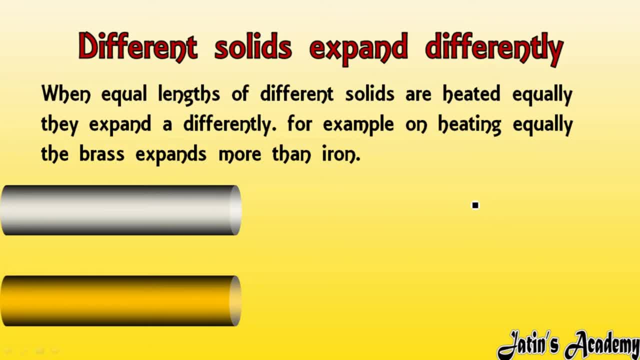 the solids. but yes, if we are having different solids, different solids will expand differently. for example, this: i am having the wire or the rods of the two material- for example, this is a iron material, okay, and this is brass material- whenever i am going to heat these both materials, these 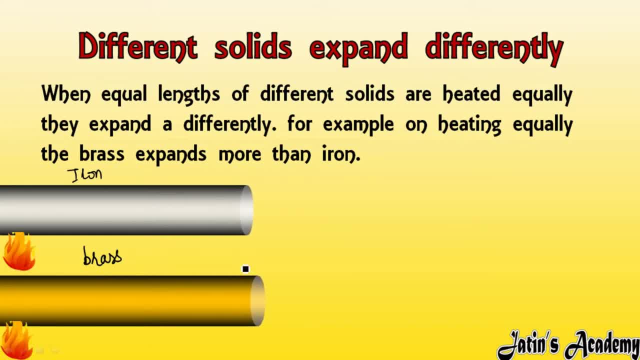 both solids are having the same length and same amount of heat. i am going to give to this both the materials. you will observe that brass will expand more as compared to iron. so thermal expansion also depends from material to material or solid to solid. so this thermal expansion in 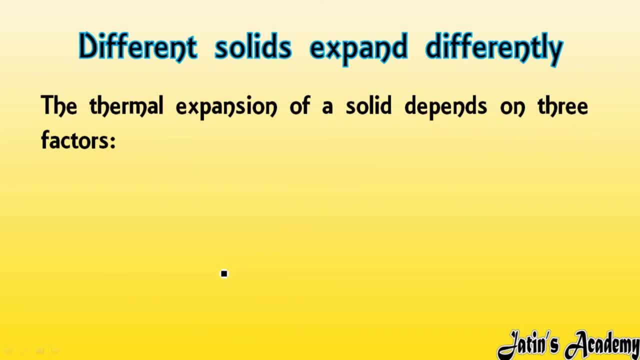 a solid depends upon three factors. what are that three factors? see carefully. firstly, it is going to depend upon the original dimensions of the solid, that what is the original length, or what is the original area, or what is the original volume of the solid. in that also it is going. 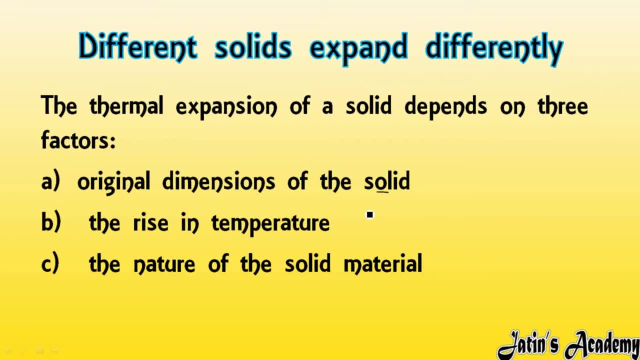 to depend the thermal expansion. and second, we are having rise in temperature. that, how much temperature we are giving in order to expand it, that is also the considerable fact, okay. and third, we are having the nature of solid material, as i already told in the previous slide, that thermal expansion. 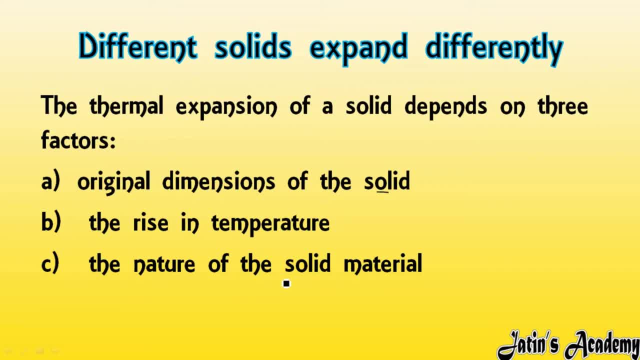 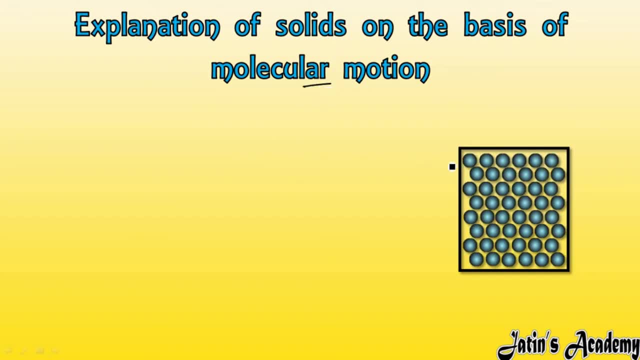 depends upon material to material. different material expands differently. now we will see that how thermal expansion of the solids are there according to its molecular motion, that how molecules move, how molecules expand. whenever we are heating any solid, for example this: i am having a solid, there is a molecular particles in the solid. okay, these are the molecules in the. 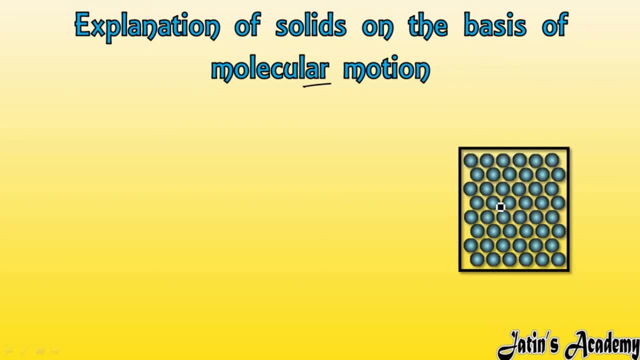 solid and the molecules of the solid are randomly moving around their mean position only or going to move to and fro about their mean position only. but whenever i am giving the heat to this solid molecule, these molecules are going to move away from each other. these molecules firstly, take the 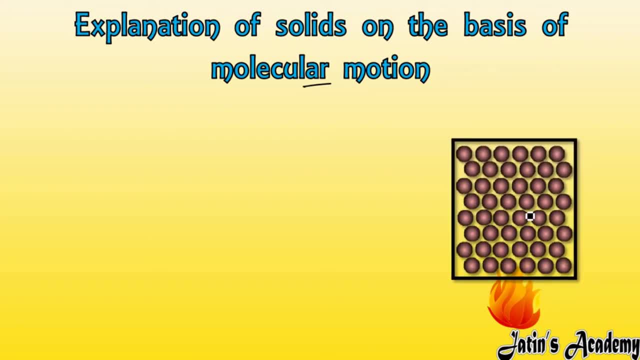 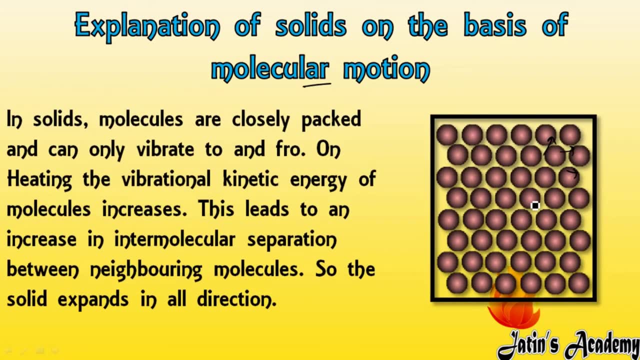 heat from the fire. after taking the heat from the fire, these molecules will strike on the walls of container. after striking on the walls of container, it will expand the size of the container. after expanding the size of the container, you will say that, yes, there is a expansion in the solid. so in 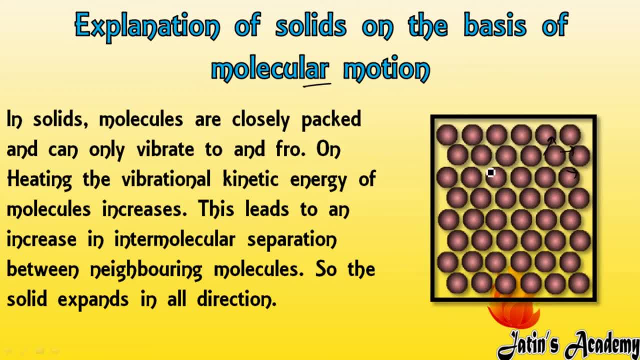 the molecules or in a solid molecules are very closely packed to each other, as we already know. in the state of matter chapter we have already discussed that there is a very compact arrangement or the tight arrangement in the solid molecules, but they are only just vibrating to and fro about. 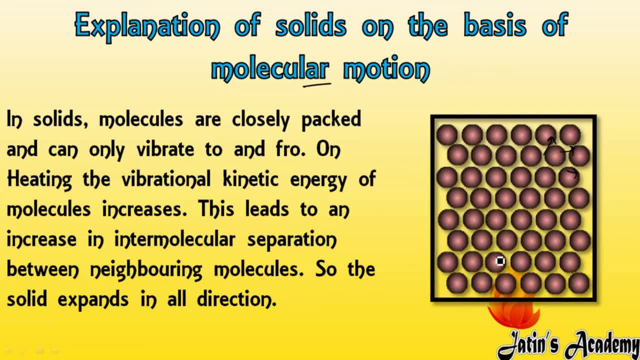 their mean position. and whenever we are going to heat the solid, whenever we are giving the heat to the solid, the vibrational kinetic energy of the solid is going to increase. means firstly they're giving the ball of energy, but now, after gaining the heat, the kinetic energy between the molecules. 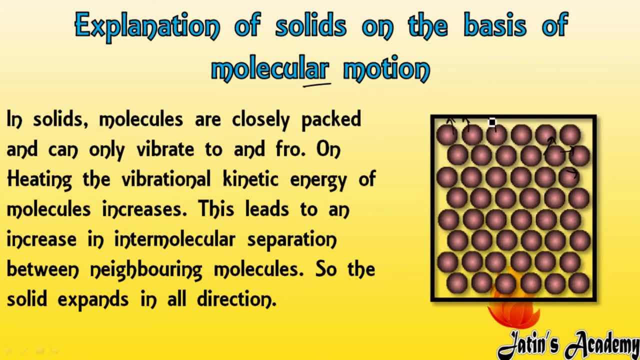 increases means whenever they are moving with the higher kinetic energy, they will push the force or they will give the pressure to the walls of the solid. whenever they are giving the pressure to the walls of the solid, they are just expanding in its size. by expanding in the size, there is a thermal 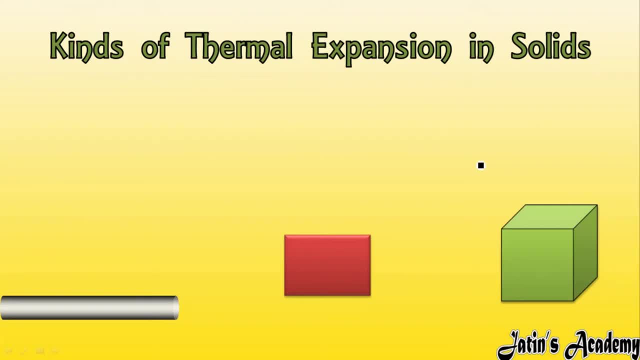 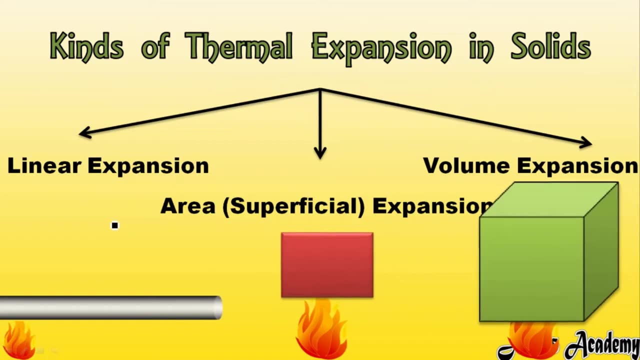 expansion by gaining the heat. so thermal expansion in solids are of three kinds. firstly, it is having a linear expansion. second, we are having area expansion. and third, we are having the volume expansion. so, one by one, we will discuss linear expansion. what is area expansion? or you can say superficial expansion, and what do you mean by? 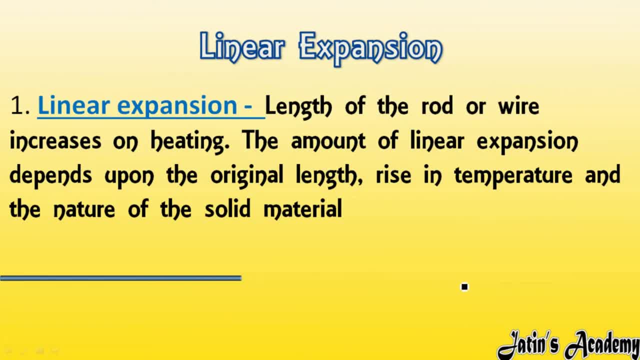 volume expansion. so very first kind of thermal expansion in solid we are having linear expansion, as a name suggests. linear linear means lengthwise means. whenever we are taking any solid which is having only its length means it is not having this much breadth, it is not having this much height. 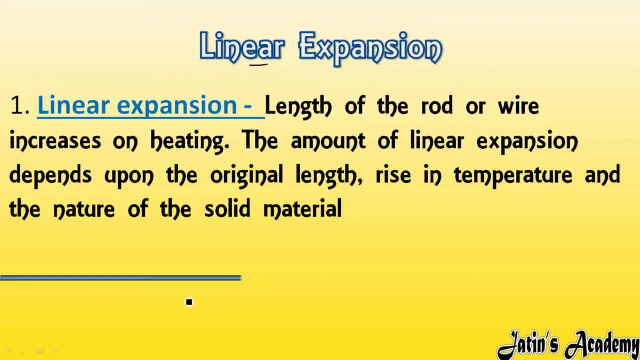 only length is there. you can say: thin rod is there or thin wire is there. okay, whenever i'm going to heat the thin rod or thin wire, it is going to expand or it is going to increase its size, so the length of the rod or the wire is going to increase on heating and this amount of the 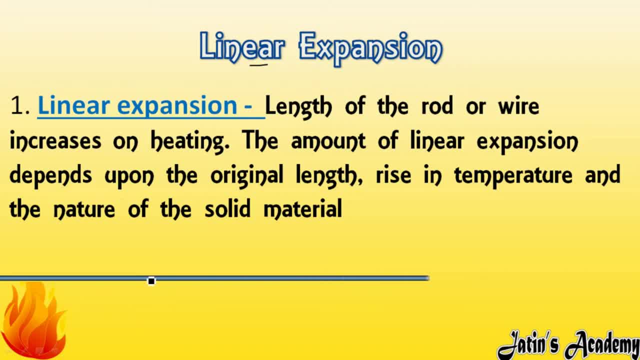 expansion depends upon the three factors. this amount of expansion depends upon three factors. what are that three factors? firstly, it is the original length. what is the previous original length of the solid or the wire? on this previous length it is also going to depend thermal expansion. accordingly, the thermal expansion will be there. second, we are having rise in temperature. how? 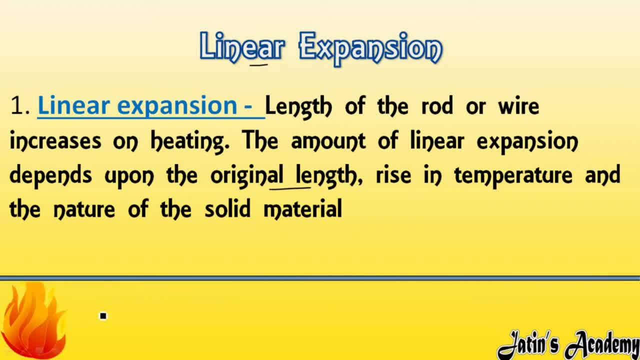 much temperature we giving in order to thermal expansion or in order to show thermal expansion. in that case also it is going to depend. and thirdly, it is going to depend upon nature of the solid material. obviously, different solid expand differently, so it is also going to depend upon the nature of the solid. 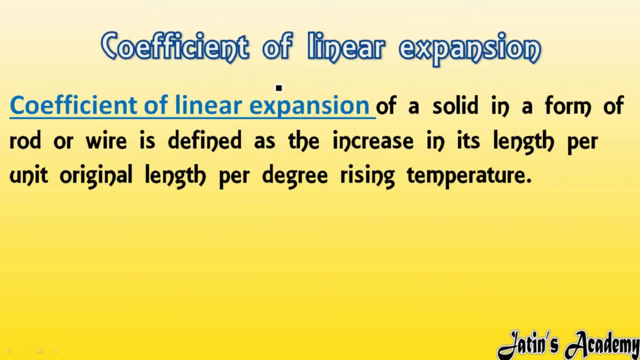 material. so now we will discuss about the coefficient of linear expansion. might be- this is very new for you- coefficient. coefficient means, for example, i am having the very thin rod, this very thin rod i am having, which is having original length, that is, l. this rod is having 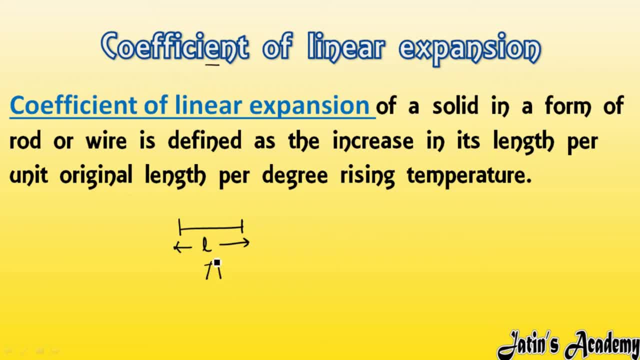 original length, that is l, and whenever i am giving the heat or temperature to this rod, after gaining the temperature or after gaining the heat, there is a expansion in the length of the rod. for example, this expansion is delta. l means, firstly, original length is l of the rod, and after 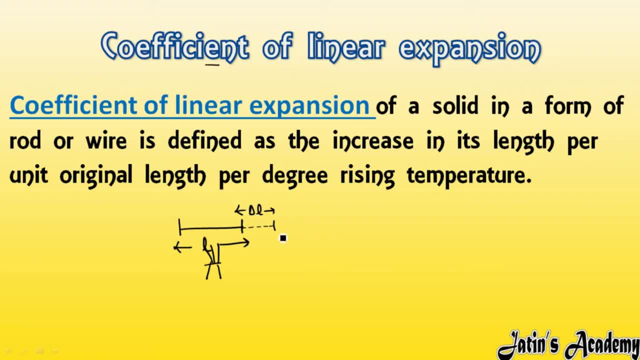 taking the heat now the after expansion. delta l is the increase in the length of the rod. okay, and for example, delta t is a temperature change in the length of the rod. delta t means a change in temperature. firstly, this rod is at the normal room temperature, but whenever i am, 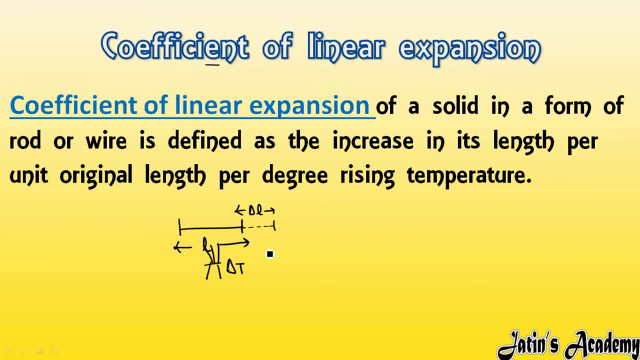 giving the heat to this length. there there is a increase in the length. after taking the heat. you can say delta t temperature is there or change in temperature is there on the rod. so this increase in length of the rod is directly proportional or going to depend upon, firstly on: 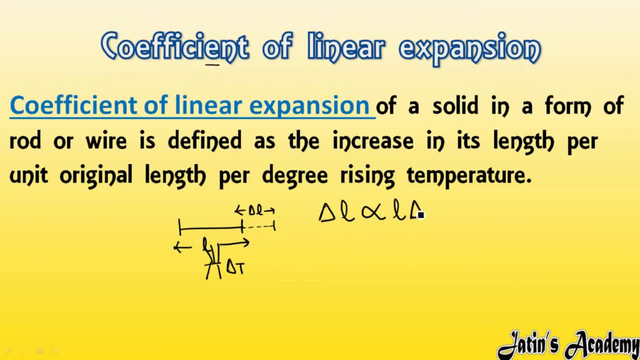 its original length, then it is going to depend upon change in temperature. whatsoever change in the length is there of the rod. that is going to depend firstly, on the original length of the rod. secondly, it is going to depend upon the amount of temperature or the change in. 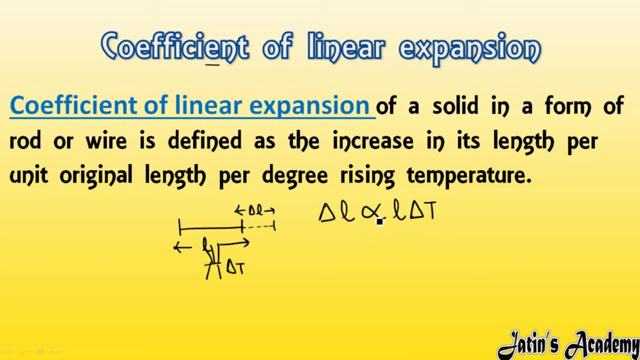 temperature whatsoever we have given. okay so, but in numericals we are not using the directly proportional sign. in that cases we are using the is equal to sign. so in order to convert the directly proportional to the is equal to sign, we have to use one kind of constant here, so delta l. 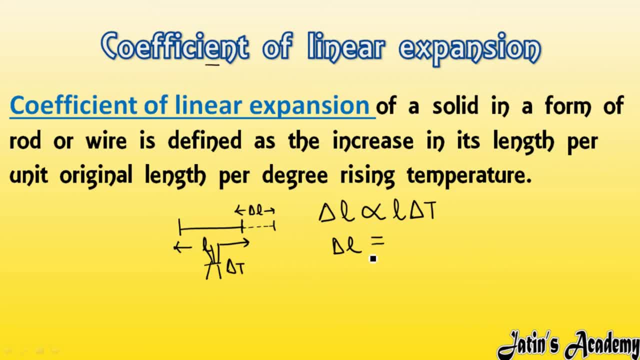 is, as such, instead of directly proportional, we are having the equals to sign. but whenever we are converting directly proportional into the equal to sign, we have to use one constant. and here, in order to use for the linear expansion, i am using one constant- is known as alpha. 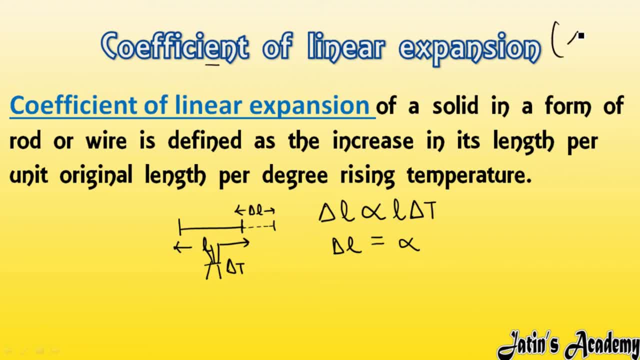 alpha is nothing but a coefficient of linear expansion. now clear: what is alpha? what is coefficient of linear expansion? so delta l is equals to alpha. l delta t is, as such, this alpha is known as coefficient of linear expansion. now i will tell you what is the definition of alpha. what is the definition? see carefully: delta l is, as such, l delta t. 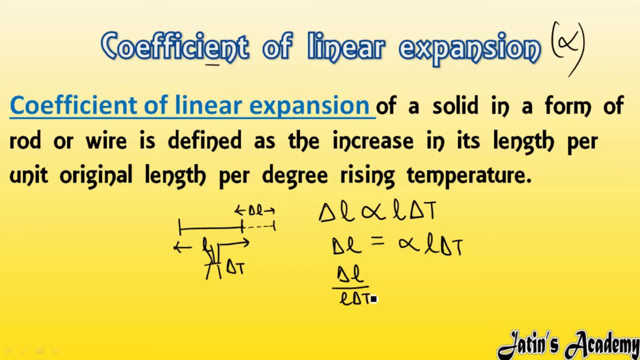 is multiplying. in that case it will go in. divide is equal to alpha as such. now see carefully what is the definition of alpha. alpha is defined as in the length of the rod per unit. original length per degree. rise in temperature. definition clear from the formula that coefficient of the linear expansion is equals to change in the length of. 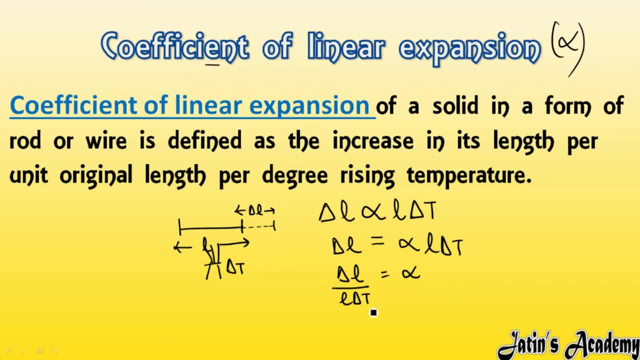 rod per unit. original length per degree. rise in temperature. this is known as coefficient of the linear expansion clear. so now we are having the SI unit of coefficient of linear expansion. what is the coefficient of linear expansion? that is alpha, okay. so now i'm going to show that what is? 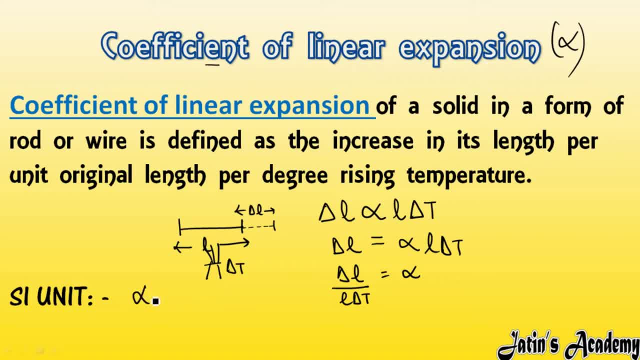 the SI unit of alpha. see carefully. as we know, alpha is equals to delta l over l, delta t. now i'm going to put the SI units of all these values. as we know here, delta l means length. what is SI unit of length? SI unit of length is meter over. we are having l is also length, length also SI unit is. 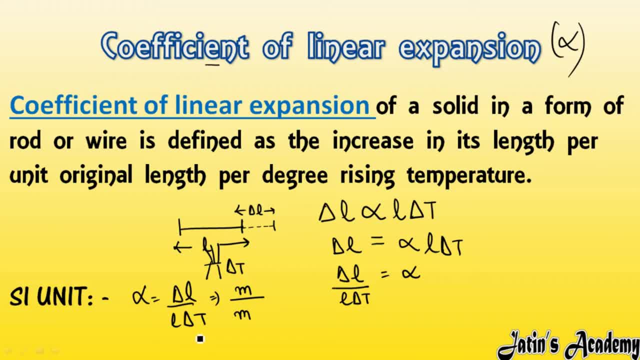 meter and delta t is what. delta t is a change in temperature. what is the SI unit of temperature? SI unit of temperature is kelvin clear. so meter cut with meter. these both units are going to cut with each other what we left with. we left with one over kelvin, one over kelvin. you can also write it like per kelvin. so what is? 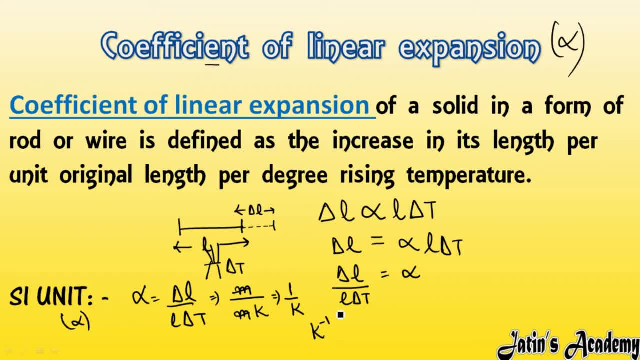 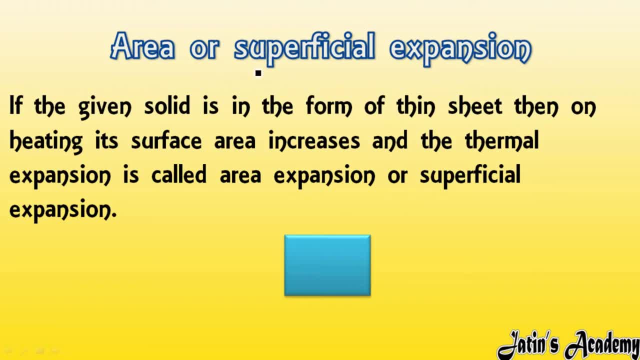 the SI unit of alpha. SI unit of alpha is, per kelvin clear. what is SI unit? so now we are having the second type of thermal expansion of solid, that is, area, or you can also say superficial expansion, as the name suggests. area in area we are going to take a thin sheet which is having the length. 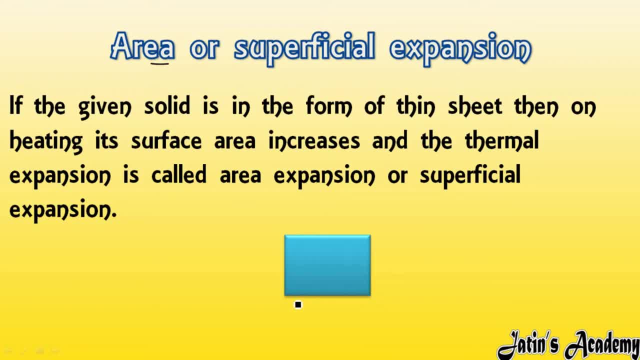 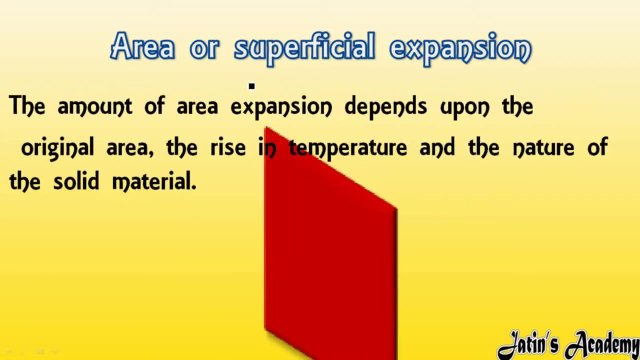 which is having the breadth also. so whenever we are having the solid in a form of thin sheet, then heating this thin sheet there is a increase in the surface area of this material. so this increase in the surface area of this material or this solid is known as area or superficial expansion. so the 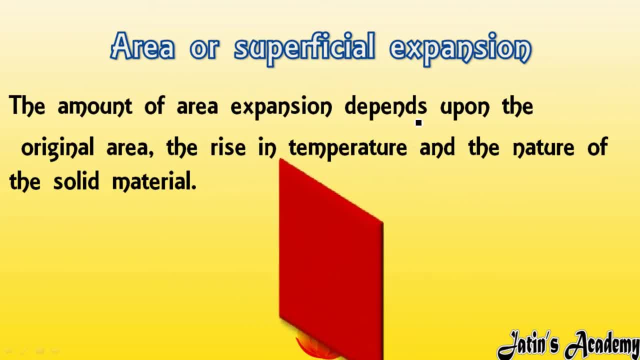 amount of area or superficial expansion is also going to depend upon the three factors. what are that three factors? that is original area, then we are having rise in temperature, then we are having nature of the solid material- whatsoever- expansion we are going to study in this chapter- either it. 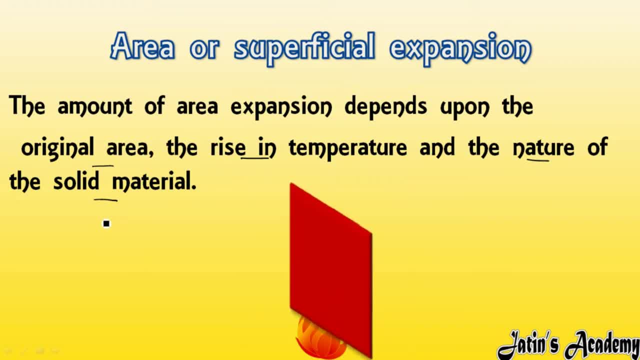 will be linear expansion, area or superficial expansion, or third, we are having the area or having the volume expansion. in each and every case, we are going to just say that all these expansion are going to depend upon three factors. that three factors are original length, original area or original volume, you can say. and second, there is a rise in temperature. and third, there 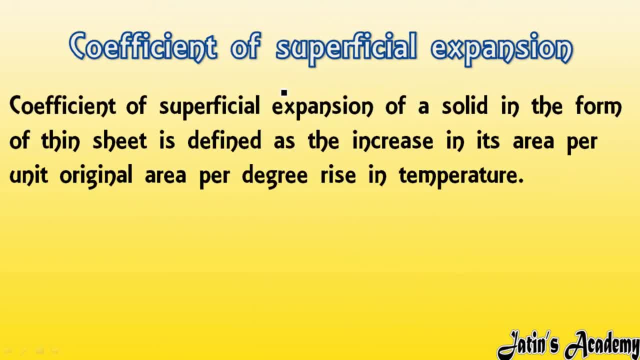 is a nature of the material used. okay. so, as we have discussed about the coefficient of linear expansion- and coefficient of linear expansion is what it is, alpha- okay, and now we are going to discuss about the coefficient of the superficial expansion, that is, area expansion. so see carefully. 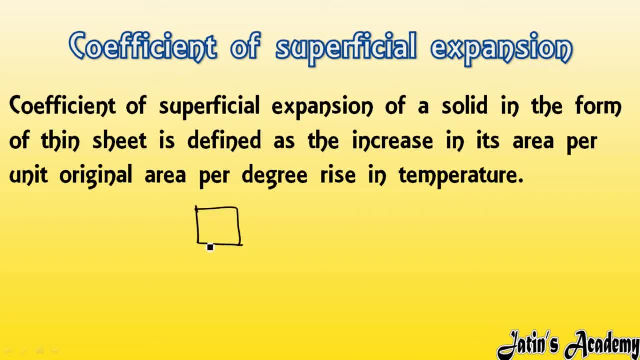 for example, here i am having a thin sheet which is having summit's length, summit spread. okay, so after giving the heat, after giving the heat, there is an increase in the area of the solid. obviously there is a thermal expansion of the solid also, firstly, let us say, that original area of the solid. 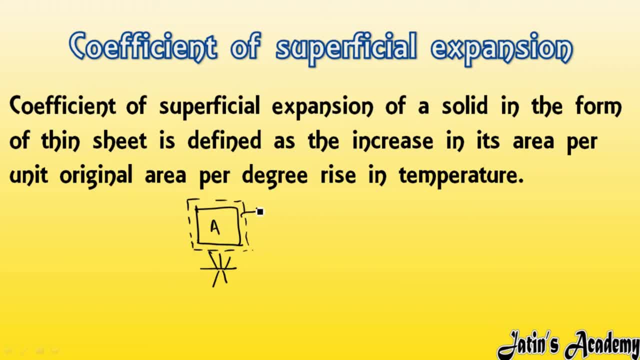 is a and after taking the heat, the change in the area is delta a. and whatsoever change in temperature is there. change in temperature generated by heat is going to be directed from willing to it and change in temperature together. that getting started and with applicable change in temperature, is delta t. Now see carefully: whatsoever there is a change in area that change. 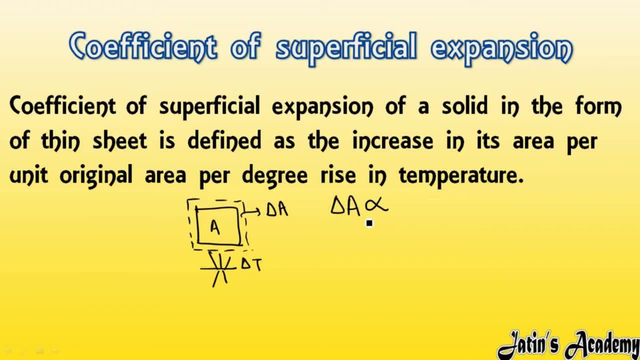 in area is directly proportional or going to depend upon two factors. that is firstly the original area, that is a, and it is also going to depend upon that. whatsoever change in temperature is there means delta a or change in area is directly proportional to original area and what is a. 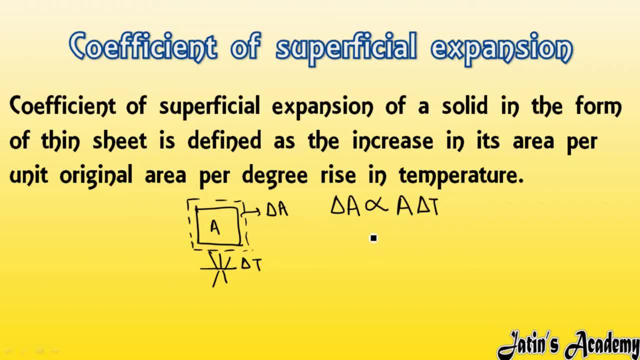 change in temperature. but in numericals we are not going to use directly proportional sign, or in any case we are not using that much directly proportional sign. we are always using the is equal to sign. so here also i'm going to convert the directly proportional to is equal to sign. 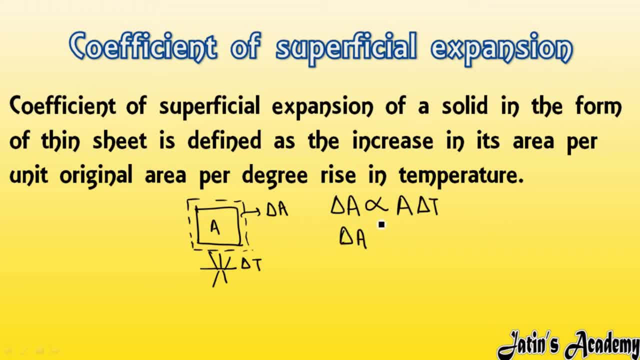 so delta a is, as such, instead of directly proportional. i'm going to use here is equal to. but yes, in order to convert the directly into the is equal to sign, i have to use one coefficient or use one constant, and here, in this case of the superficial expansion, i'm going to use one. 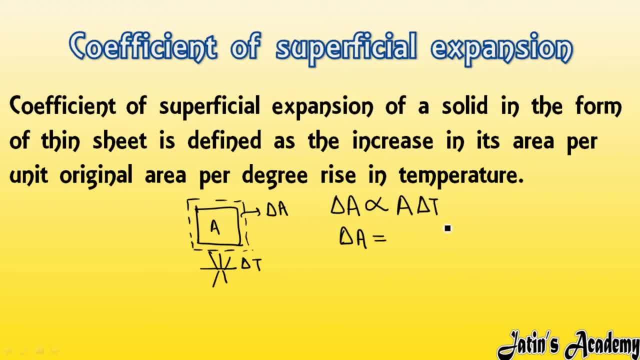 different coefficient or the different constant. that constant is known as beta. beta is what beta is, nothing but the coefficient of superficial expansion. next, a delta t is, as such. now i am going to define that. what is beta? what is coefficient of the area expansion? see carefully: delta a is, as such, over a delta t. a delta t is, as such, is equals to beta. okay, now, what is beta? or? 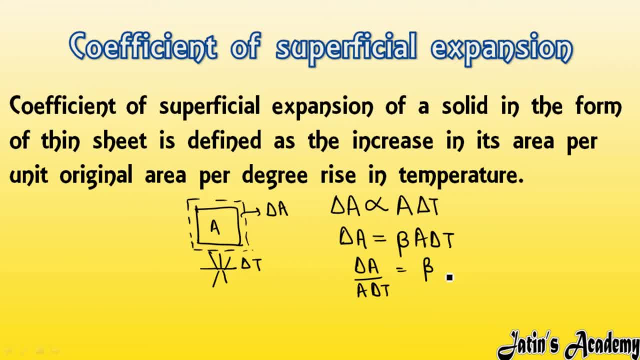 what is the coefficient of area expansion? coefficient of the area expansion is defined as change in area per unit, original area per degree, rise in the temperature. so by watching the formula only you can can just write the definition also. okay. so next we are having its SI unit, as we know, beta or 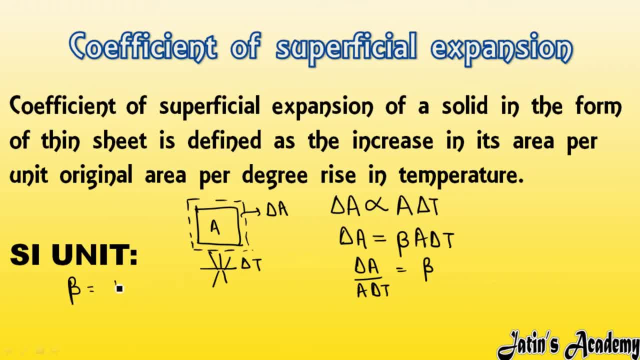 coefficient of superficial expansion is beta, that is, delta a over a delta t. okay, now just put the SI unit of the area and temperature. what is the SI unit of area? SI unit of area is meter square over. SI unit of area, again, is meter square. delta t means change in temperature, temperature SI unit. 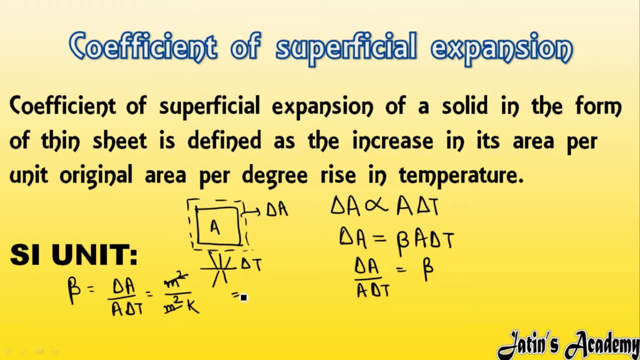 is kelvin. okay now meter square, cut with meter square, what you are left with? you are left with one over kelvin. so one over kelvin is nothing but per kelvin. so what is the SI unit of coefficient of area expansion? SI unit is, per kelvin, same as the coefficient of the linear expansion. 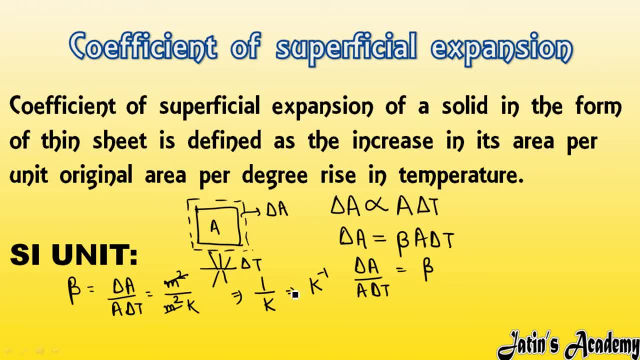 means the coefficient of linear expansion, SI unit of coefficient of linear expansion, SI unit of coefficient of superficial expansion, as well as SI unit of the volume expansion. they all are same, only that is per kelvin. SI unit of alpha beta, and in the volume expansion you will. 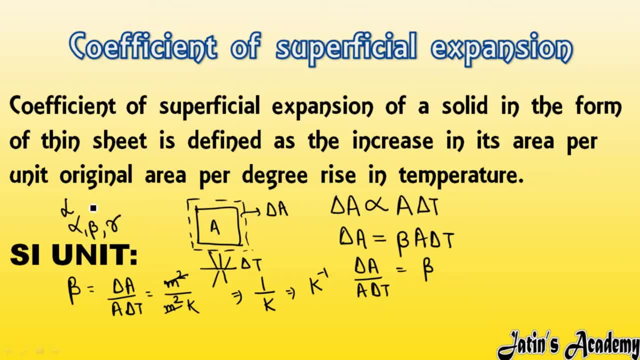 say that it is gamma, okay, this is a linear expansion. and in the volume expansion you will say that it is a linear expansion. this is area expansion and this is volume expansion. all the SI units are same, only that is per kelvin. and whatever other unit we are using. other unit is: 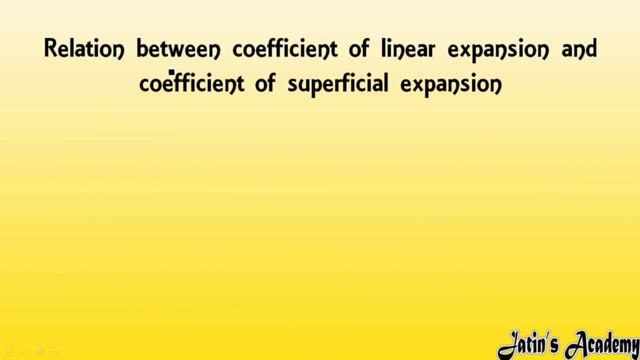 per degree celsius. so next topic: we are having relation between coefficient of linear expansion and coefficient of superficial expansion. as you know, coefficient of linear expansion is nothing but alpha and coefficient of superficial expansion is beta. now we are going to see the relation between alpha and beta. so relation is like this: beta or coefficient of superficial expansion. 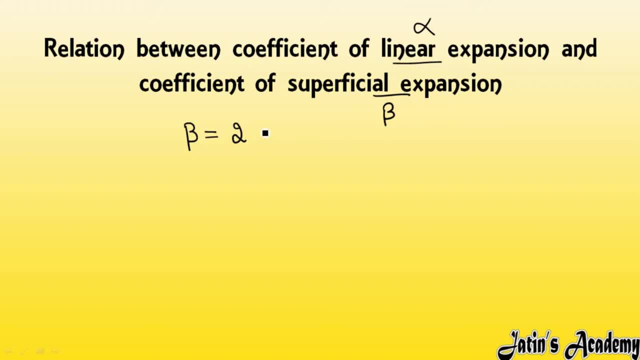 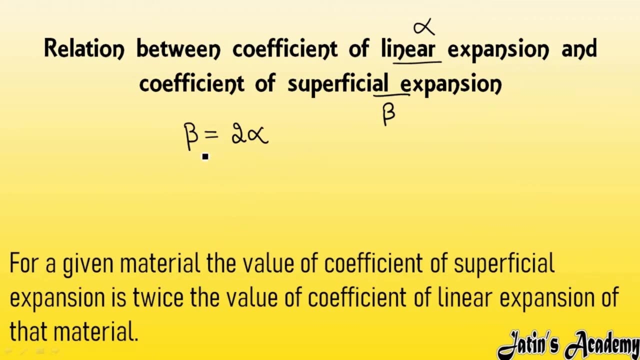 is equals to twice, or coefficient of linear expansion. that is, beta is equals to 2 alpha. and now how in relation came that? you will do in the higher classes, okay. so here we are having the definition of this relation between alpha and beta for a given material, the especialื่ imgq. 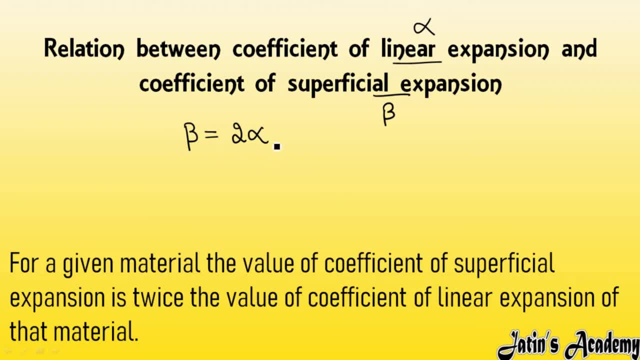 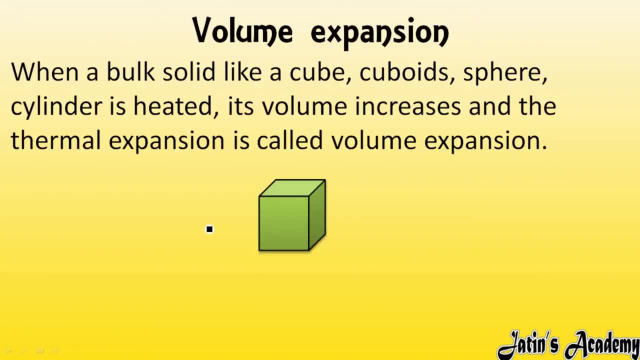 of coefficient of superficial expansion is: is means is equal to twice of the value of coefficient of linear expansion of that material. okay, this is a relation between alpha and beta. so now we are having that is known as volume expansion. what do you mean by volume expansion? as a name suggests volume. 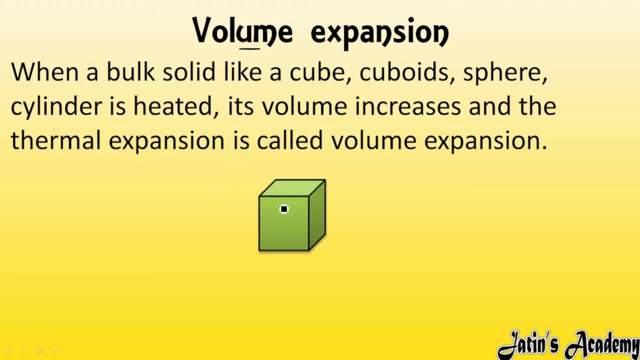 volume means whenever we are taking any bulk solid. bulk solid means either we are taking cube, cuboid, sphere, cylinder whenever we are having any bulk solid and we are going to heat that solid, which is having its length, breadth as well as its height also whenever we are heating it. so there is 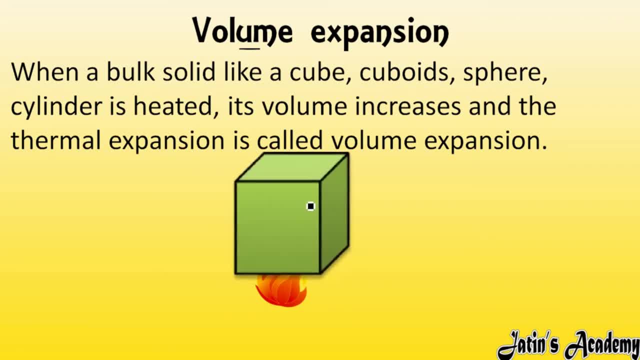 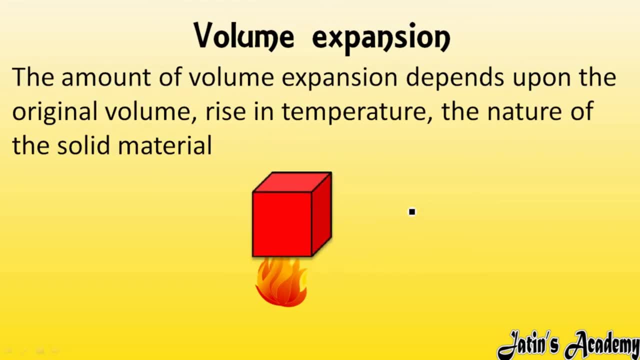 an increase in the volume of the material, and this expansion, or this thermal expansion, is known as volume expansion. so again, this volume expansion is going to depend upon the three factors. what are that three factors might be? now you are knowing. first factor is original volume. second factor is rise in the temperature. and third, we are having the nature of the solid material. here 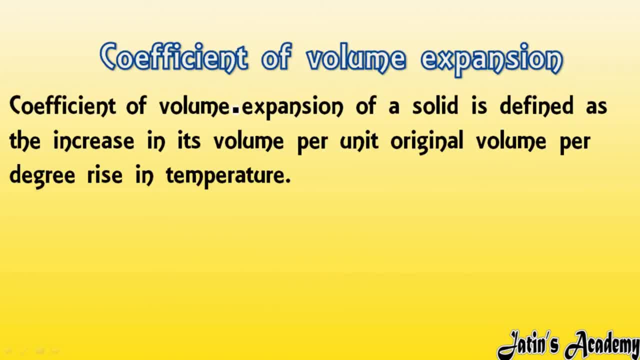 we are having the coefficient of the volume expansion. see carefully: what is the coefficient of volume expansion? for example, here i'm having the volume which is having its original volume, v, before giving heat. the original volume of solid is v, but whenever i'm giving the heat to this volume, 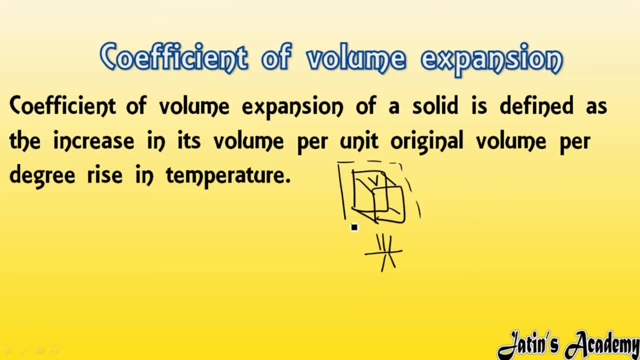 after taking the heat, for example. now the volume is delta v, now change in volume after thermal expansion is delta v and temperature is delta t. so this change in volume is directly proportional or going to depend upon two factors. firstly, it is the original volume, then we are having the change in temperature. so again, instead 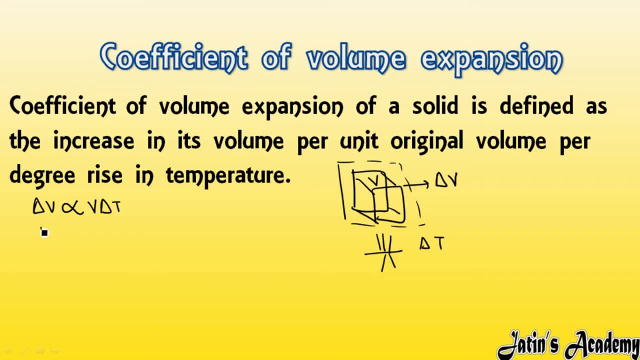 of directly proportional, we are going to use the- is equal to sign, so delta v is equals to. here also i have to use one constant and, as we know, in the linear expansion you have used alpha. in the coefficient of area expansion you have used b, and in the linear expansion you have used b, and in the 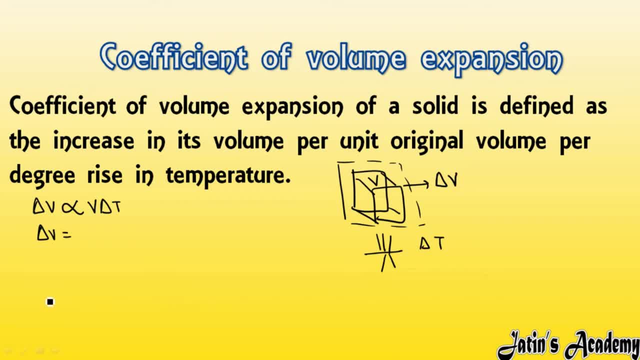 beta. and now, in the volume expansion, or the coefficient of volume expansion, you are going to use one constant, and that constant is known as gamma. so it is gamma. v, delta, t is as such. so what is gamma? gamma is nothing but coefficient of volume expansion. so now we are going to define the 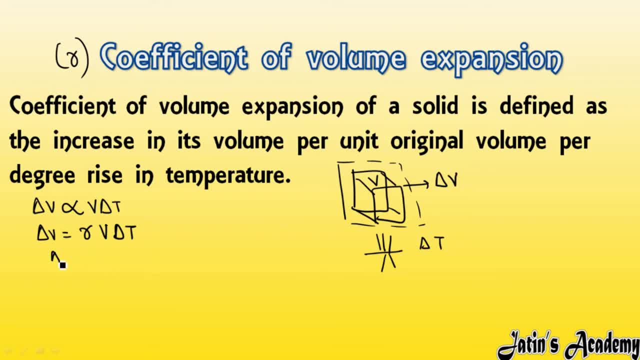 coefficient of volume expansion, that is gamma. delta v is, as such, over v. delta t is equals to gamma. what is the definition of gamma? gamma means change in volume per unit, original volume per temperature. okay, this is the definition of the gamma. now we will see the si unit for the gamma. what 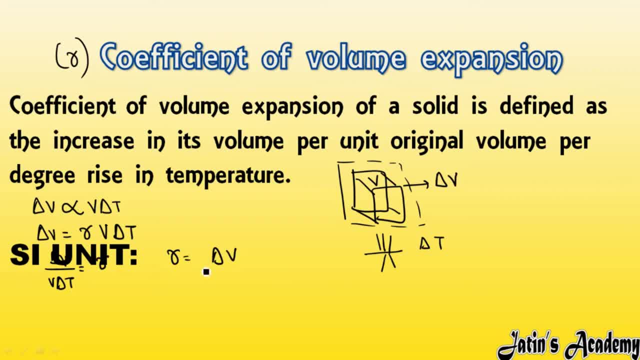 is the si unit. as we know, gamma is equals to delta v over v, delta t. so what is the si unit of volume? si unit of volume is meter cube. over again, volume is there meter cube and delta means change in temperature, that is kelvin. so meter cube cut with meter cube. again we are having one over kelvin one. 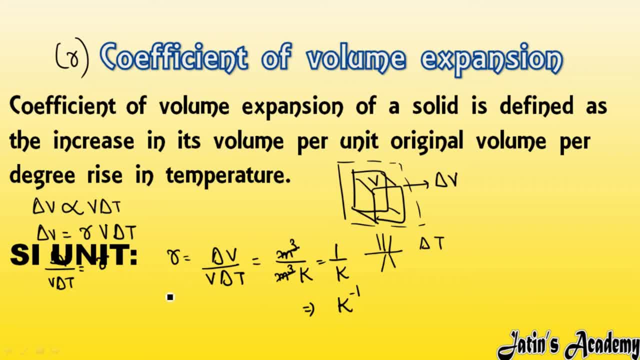 over kelvin is nothing but per kelvin. so si unit of gamma, or the coefficient of volume expansion, is per kelvin. if you want to write in the degree sequence, you can write in the degree sequence from other unit. other unit is per degree celsius, clear, always note one thing: that we are not going. 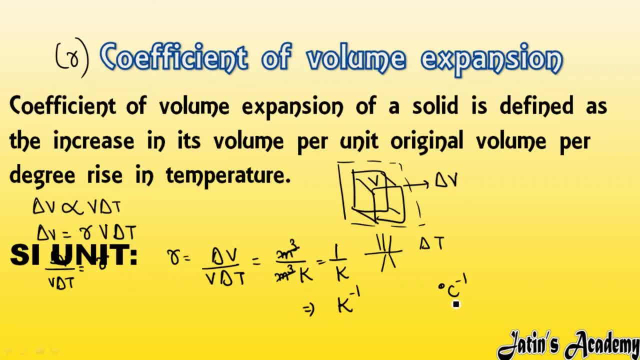 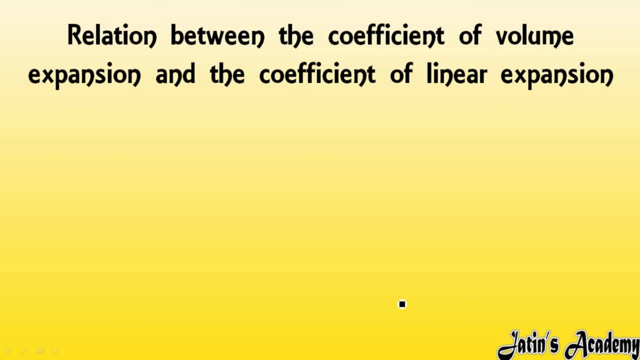 to use degree with the kelvin only degree we are using with the degree celsius. okay, kelvin, we are going to simple write kelvin. so now we are having the relation between the coefficient of volume expansion and the coefficient of linear expansion. as we know, coefficient of volume expansion is: 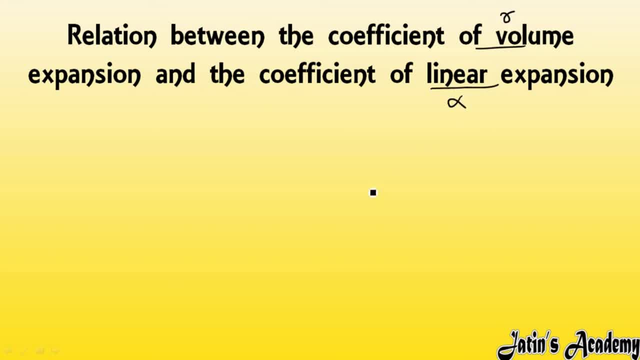 gamma and coefficient of linear expansion is alpha. what is the relation between gamma and alpha? relation is like this: gamma is equals to three alpha means for the given material coefficient of the volume expansion is thrice the coefficient of the linear expansion. okay, and one thing more in exams question will come like this: also that what is the relation between? 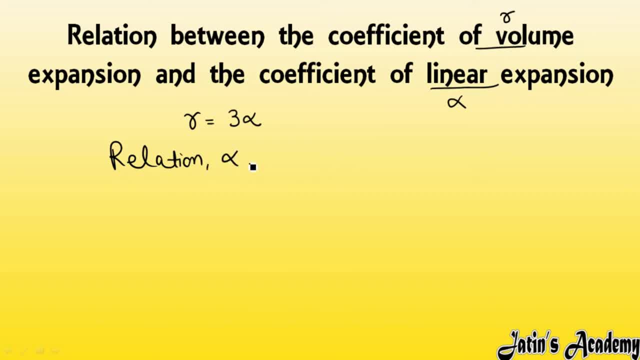 what is the relation between alpha, beta and gamma? this all relation we have to write relation is like this: gamma is equals to three by two. beta is equals to three alpha. this relation you can note it down. whatsoever derivation is there that you will do the higher classes, just note it down. 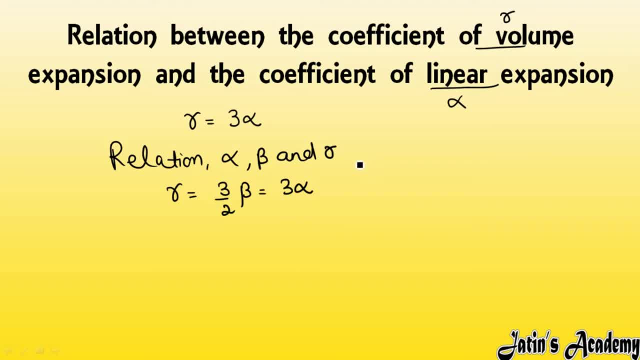 between alpha, beta and gamma. all the coefficients of the linear area and volume expansion, gamma is equals to three by two. beta is equals to three alpha. and if question will come like this that what is the ratio of ratio of alpha, beta and gamma, then its ratio is one ratio two, ratio three. 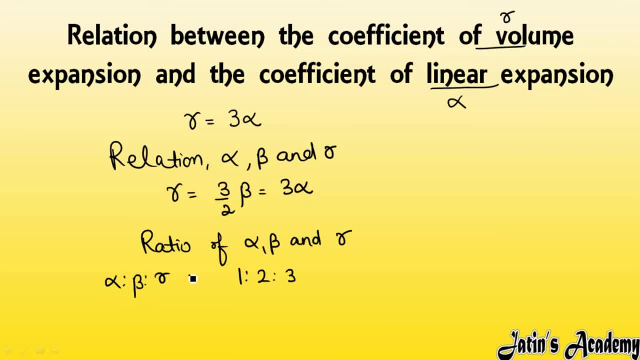 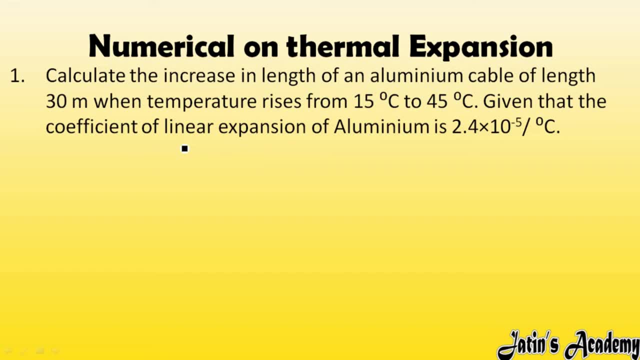 means alpha ratio, beta ratio, gamma is one ratio, two ratio, three. this also you have to learn in accordance to the exam point. so now we are having the numericals and in the numerical we will use the three formulas. first formula we will use for the alpha: alpha is equals. 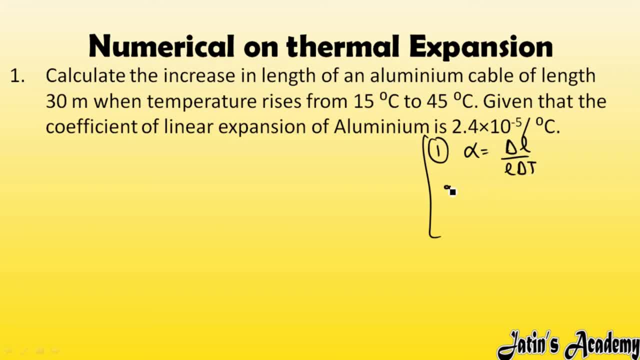 to delta l over l delta t. secondly, we will use for the beta. beta is equals to delta a over a delta t. and thirdly, we will use for the volume, that is gamma. gamma is equals to delta v over v delta t. okay, so now let us see the numerical calculate the increase in length. increase in length means: 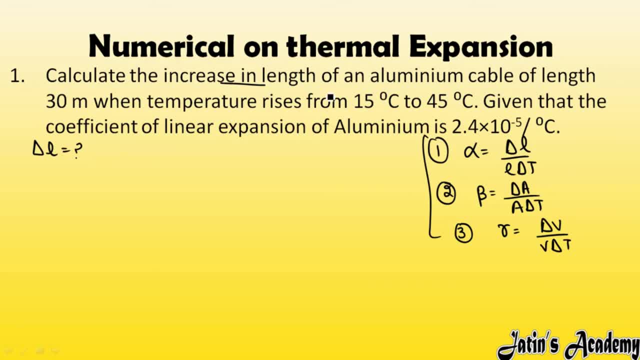 delta l we have to calculate of the aluminium cable of length 30 meter and original length is equals to delta l by сос. in addition, at 50 degree Celsius increase in length equals to delta a over a delta a minus 25 degree Celsius, minus 30 degree Celsius. okay, so what is the difference between? 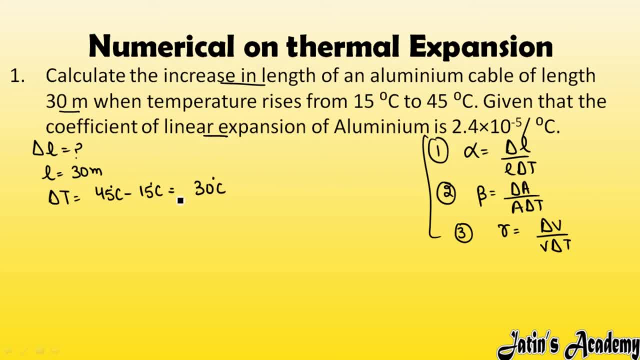 this gema and gamma values. when the temperature rises from this to this, change in temperature is given to us means temperature rises from 15 degree Celsius to 45 degree Celsius. so change, we will calculate the change means 45 degree Celsius minus 15 degree Celsius, it will give you 30 degree Celsius. okay, given that the coefficient of linear expansion, what is the coefficient of linear expansion? that is alpha? it is given to us got coefficient of linear expansion that is alpha. 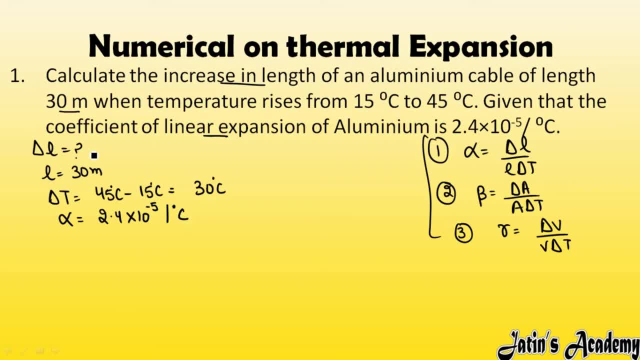 minus 5 per degree celsius. we have to just calculate delta l. how we'll calculate delta l? by using first formula of the alpha. so, as we know, alpha is equals to delta l over l delta t. so just put the values: alpha value is 2.4 into 10, to the power minus 5 delta l. we have to calculate. 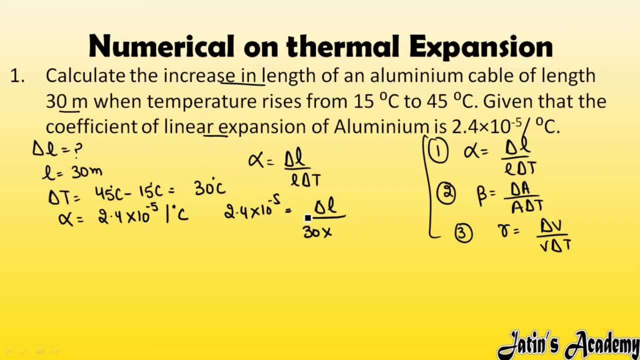 over l. value is 30. multiply change in temperature is 30, so it will be 2.4. 10 to the power minus 5 is equals to delta l over 30. multiply 30 means 900, so 900 is in divide. here it will go in. 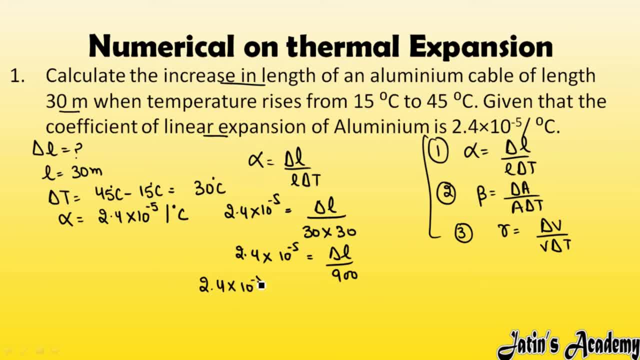 multiply 2.4, multiply 10 to the power minus 5, multiply 900 is equals to delta l. so multiply 900 with 2.4 will give you 160 into 10 to the power minus 5 is equals to delta l. okay, so here. 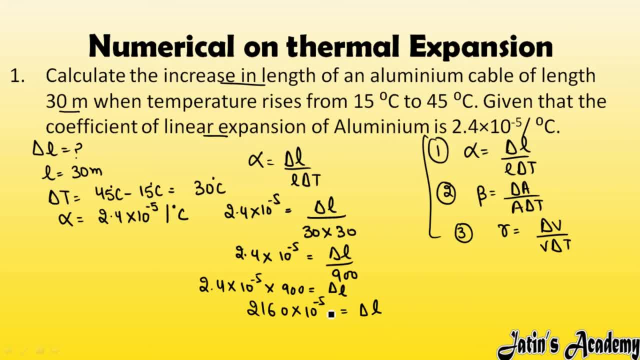 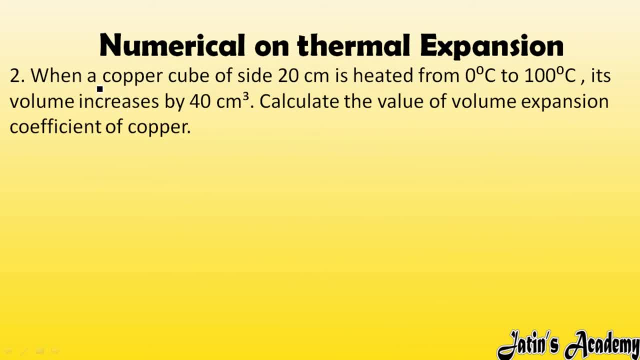 you can write l. l means a change in length. change in length means here we are having meter. this is the value of the change in length. so now we having second numerical. in second numerical we are given with when a copper cube of side 20 centimeter side of cube is given to us. side of cube is equals to 20 centimeter is heated from. 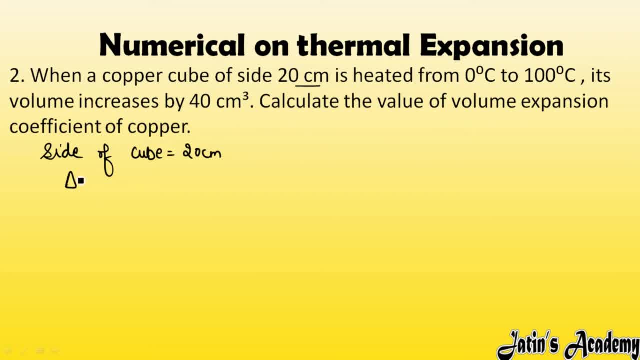 0 degree celsius to 100 degree celsius means delta t or change in temperature. is there 100 degree celsius minus 0 degree celsius? that is nothing but degree celsius. its volume increases by 40 centimeter cube. volume increases means change in volume is given to us. that is 40 centimeter cube. 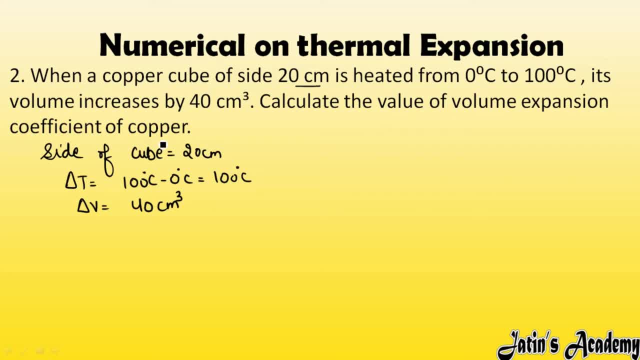 calculate the value of the volume. expansion coefficient of the copper means gamma value. we have to calculate. so in order to calculate the gamma value, first of all we need delta v, delta v. we are having over v, delta t v value. we are not having the volume. we are not having. we 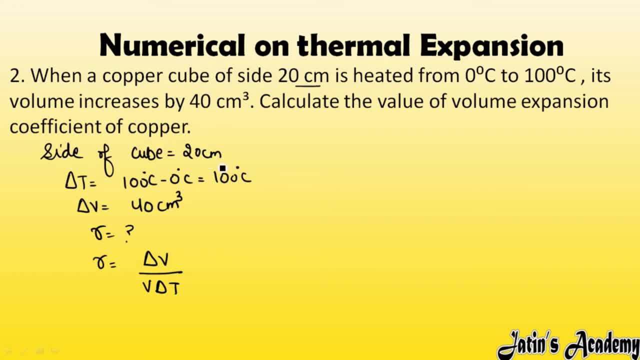 are just having the side of the cube. from the side of cube. can you calculate the volume of cube then? obviously, yes, volume of cube is equals to side cube. that is side cube. that is nothing. but side is 20 cube. 20 cube will give you 8000 centimeter cube. 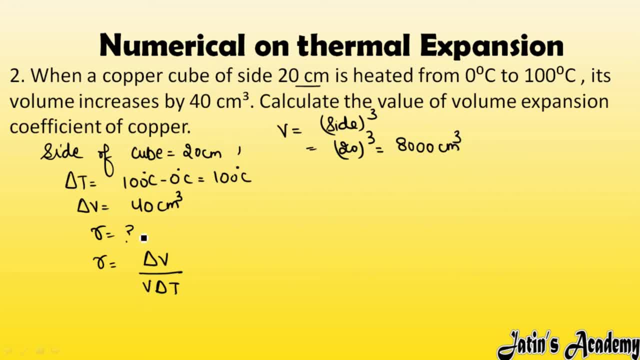 so delta v is there, v is there and delta t is also given to us. so calculate the gamma. so gamma is equals to delta v. delta v is given to us, 40 over v. v is 8000. multiply then we are having change in temperature. that is 100. so 0 cut with 0, then we are having 2. here it is 5, then we are having 1. 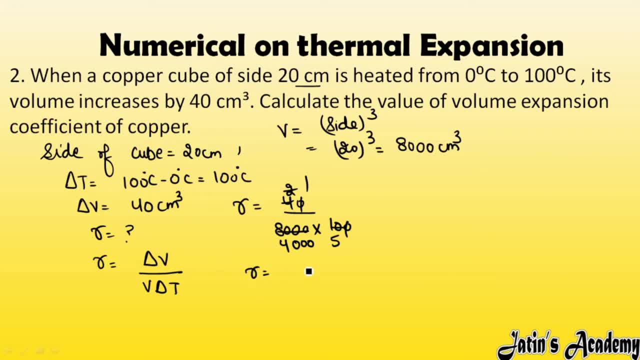 here it is we are having: 4000 gamma is equals to 1 over 20000. okay, 1 over 20000 means 5 into 10th is power minus 5 per degree celsius. this you will get as a value of the gamma. so now we are having 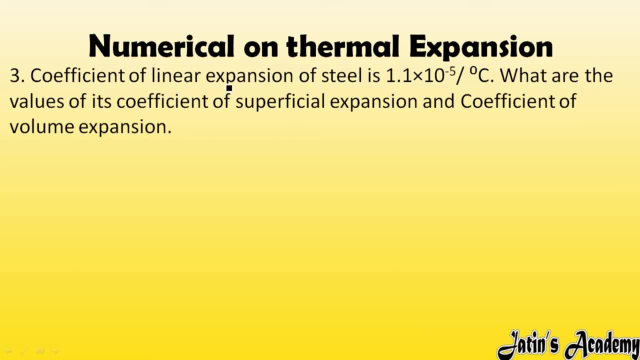 third numerical in third numerical we are given with, coefficient of the linear expansion of steel is 1.1. 10th is power minus 5 per degree celsius. so coefficient of linear expansion is given to us means alpha is given to us, 1.1, into 10th is power minus 5 per degree celsius. what are the values of? 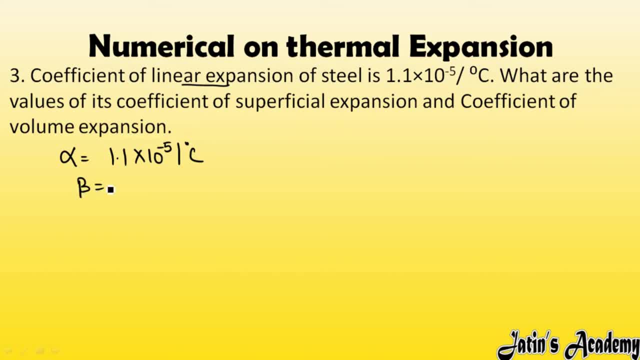 coefficient of superficial expansion- beta, we have to calculate- and coefficient of volume expansion- gamma we have to calculate. as we know, relation of beta in terms of alpha. that is, beta is equals to 2, alpha just put the values. beta is equals to 2 multiply alpha is what? 1.1 into 10 to the power minus 5, so beta will be 2.2 into 10 to. 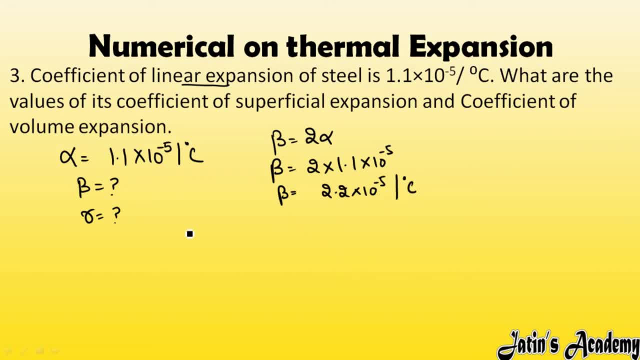 the power minus 5 per degree celsius. so now we have to calculate gamma. gamma is what gamma is equals to 3 alpha. so put the values: gamma is equals to 3 multiply what is alpha. alpha is 1.1 into 10 to the power minus 5. so solve it. gamma will be 3.3 into 10 to the power minus 5 per. 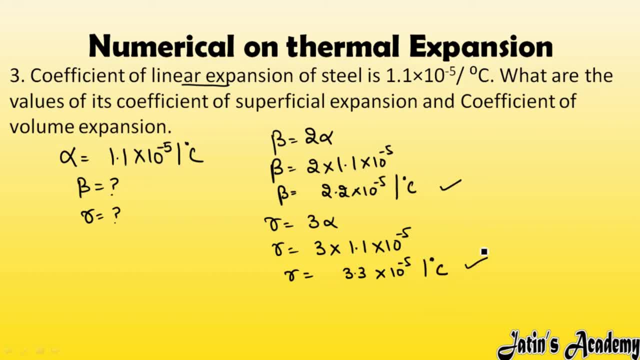 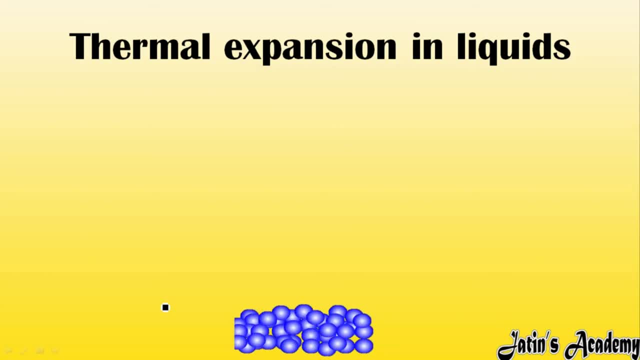 degree celsius. these are the value of beta and gamma. that is nothing but coefficient of superficial expansion and coefficient of volume expansion. so now we are going to start with thermal expansion in liquids. as we know, each and every state of matter- either it is solid liquid or gas- there. 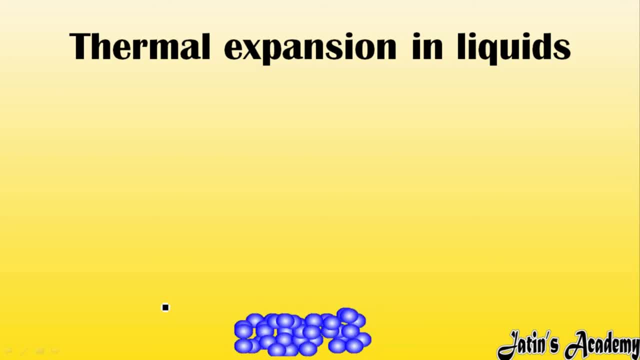 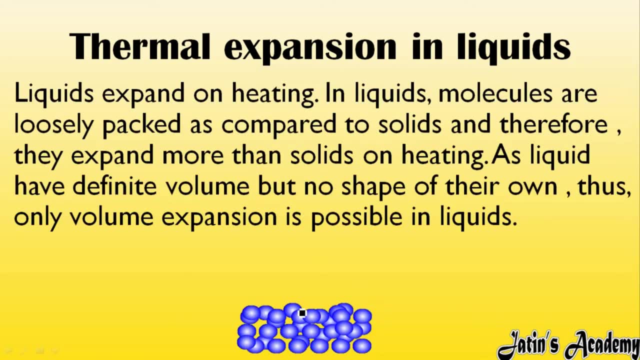 is always a thermal expansion whenever we are giving the heat to either solid liquid or the gas, for the liquid also. liquid also expand on heating. okay, but in liquids molecules are loosely packed as compared to solid. molecules of the liquid are loosely packed so therefore they expand more as compared to solid, as in solid, particles are very 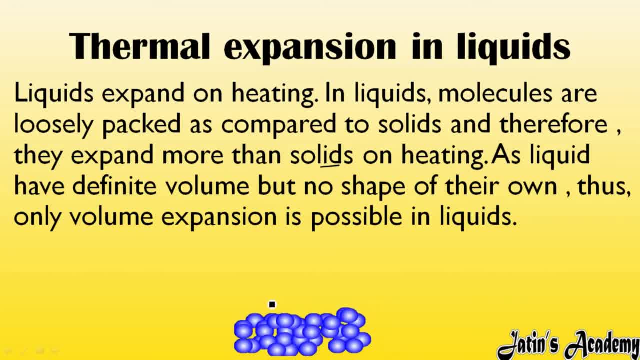 close to each other and they need very much energy in order to lose their intermolecular force of attraction. but in the liquids particles are already having less intermolecular force of attraction. so by gaining less energy, only they are just moving or they are just showing more. 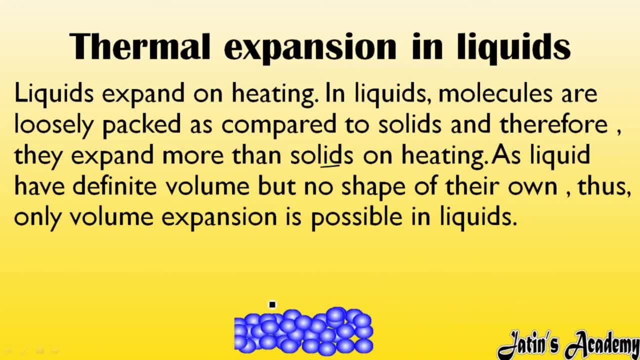 thermal expansion okay, but, as we know, liquid are having the definite volume, but liquid are not having the definite shape means we can easily change the shape of the liquid. thus, by having only its definite volume, liquids can only show volume expansion because they are not having the definite 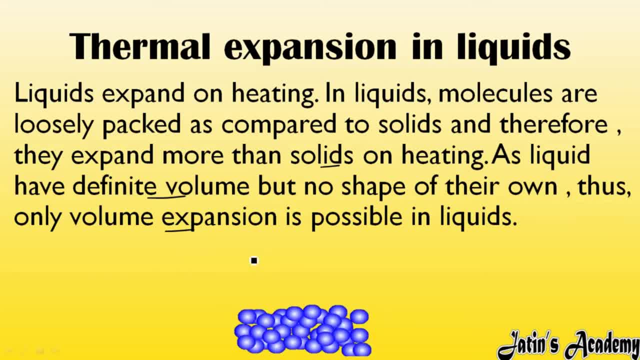 shape if they are not having its proper length, proper breadth, they are not going to show any linear expansion, they are not going to show any area expansion, they are just going to show its volume expansion because they are just having their definite volume. no definite shape is there. 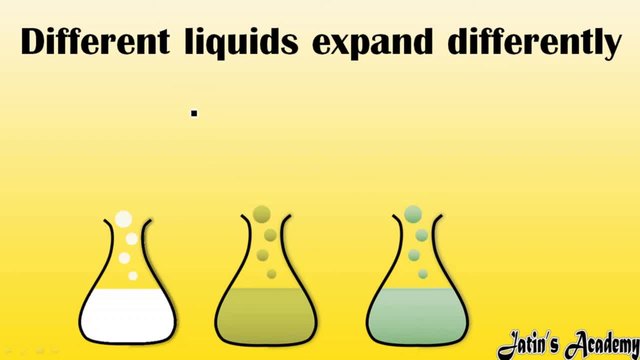 so now we are having next topic: that different liquids expand differently. as different solids are expanding differently, in the same way, different liquids also expand differently. for example, in this beaker i'm having three different liquids and whenever i'm going to heat the liquids, same amount of heat, i'm going to give the three all liquids. these liquids also expand differently. 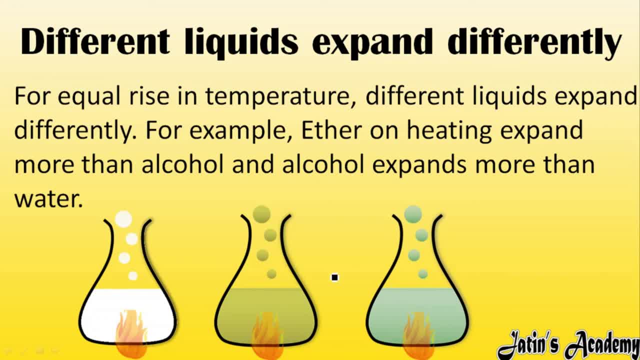 for equal rise in temperature, different liquids were going to expand differently. for example, in the first beaker i'm having ether, in second beaker i'm having alcohol and in third beaker i'm having water. okay, so in different beakers i'm having different liquids, but by giving 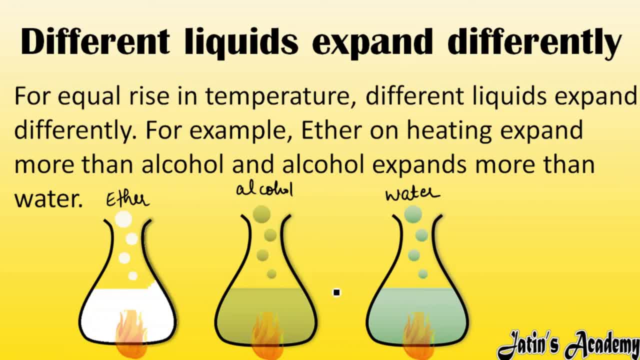 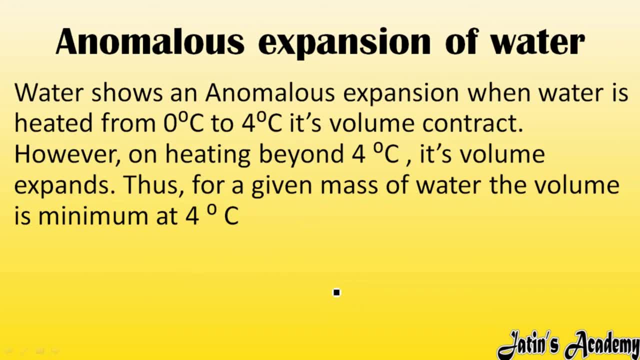 the same amount of temperature. ether will expand more as compared to alcohol and least there is expansion in the water. okay, next topic: we are having anomalous expansion of water only little bit. topic we are having in the eighth standard of anomalous expansion in water. proper study you. 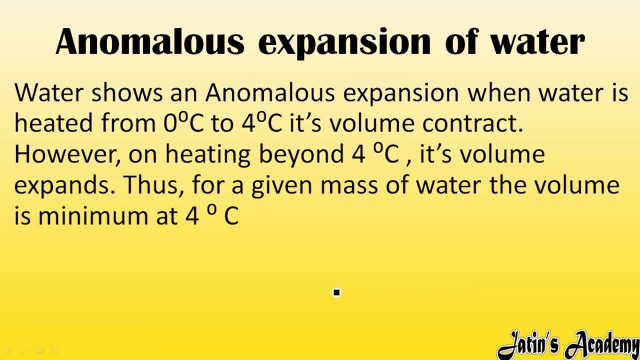 will do in the higher classes. so what do you mean by anomalous expansion in water? see carefully, actually water show. anomalous expansion means whenever water is heated from zero to four- in between zero to four degree celsius, its volume contracts. but whenever we are giving heat beyond, 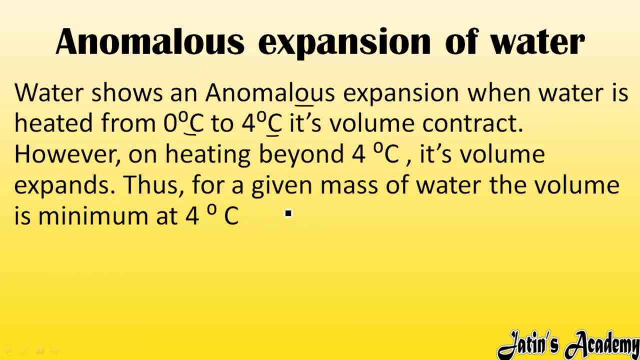 four degree celsius, then its volume going to start expanding, then it is going to show the expansion. so by the given mass, the minimum temperature, whatever we have to give in order to show the thermal expansion by water. that minimum temperature is four degree celsius and this theory is known as 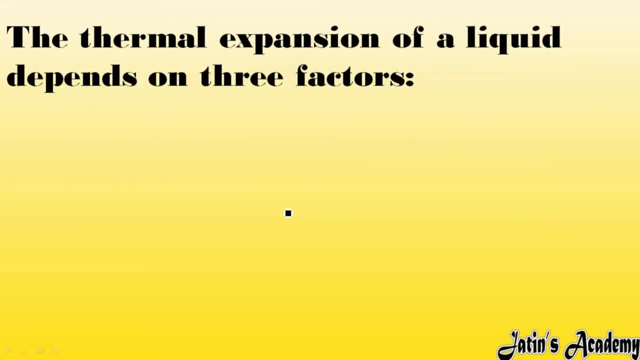 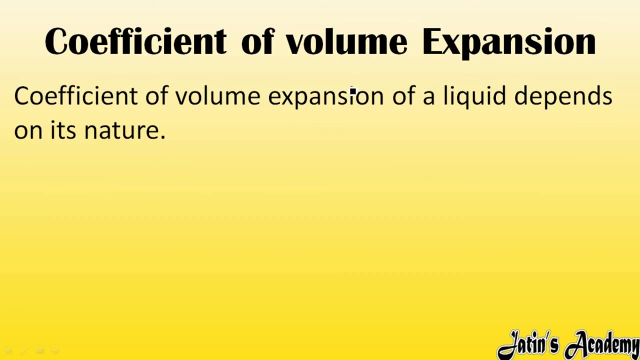 anomalous expansion of water. so this thermal expansion of liquid is also going to depend upon three factors. and what are that three factors? see carefully: firstly, it is original volume of liquid, then we are having rise in temperature and third, we are having the nature of the liquid used. so, as we have already discussed, that volume is only having its. 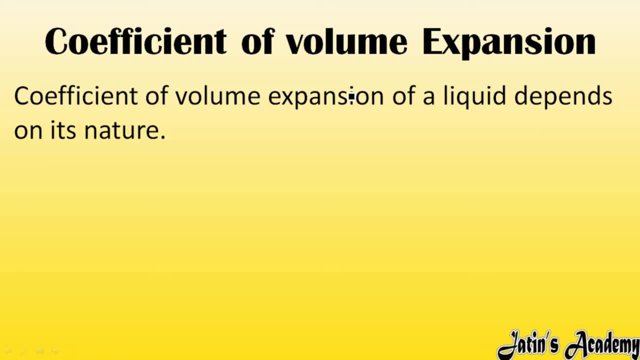 definite volume, but it's not having any definite shape. that is why, in this liquid expansion, we will just discuss about the coefficient of the volume expansion, as we already know that, for example, here we are having beaker and in this beaker water is there. firstly, the volume of the water is v, but 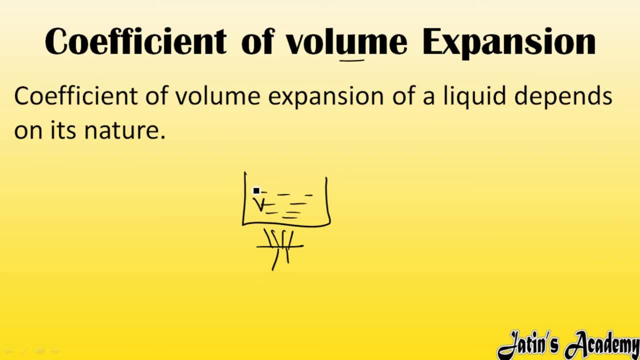 whenever i'm giving the heat or temperature to this water, there is a change in the volume. so this change will be delta v. okay, so here it will be delta t temperature. so this change in volume is going to depend upon two things, that is, firstly, original volume of the liquid. then we are. 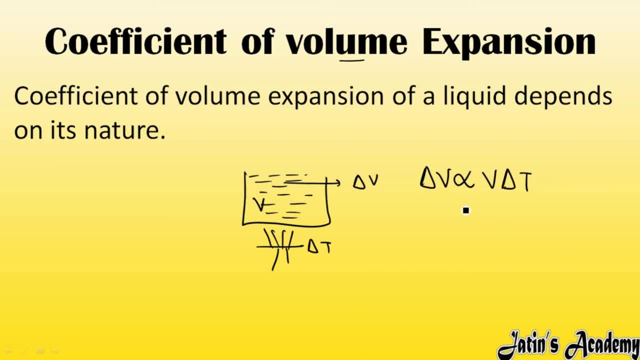 having change in the temperature. but instead of directly proportional we have to use the ist to sign the same delta. v's as such is equals to in volume expansion same. we are going to use the gamma, then v delta when we are having linear alpha for the superficial beta and for the volume either. 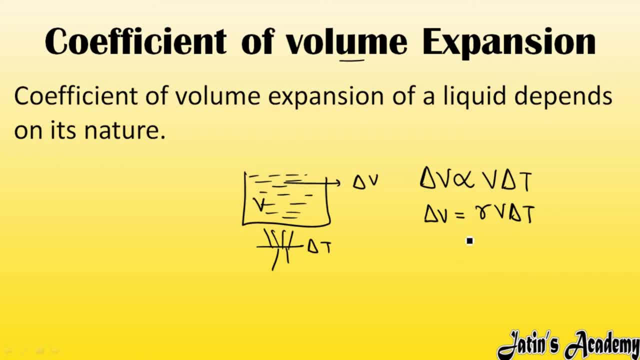 it is for the solid, either it is for the liquid or for the. we are going to use the same coefficient, that is gamma, and then we are having V, delta T as such. okay, then we are having delta V over V. delta T is equals to gamma, means coefficient of volume. 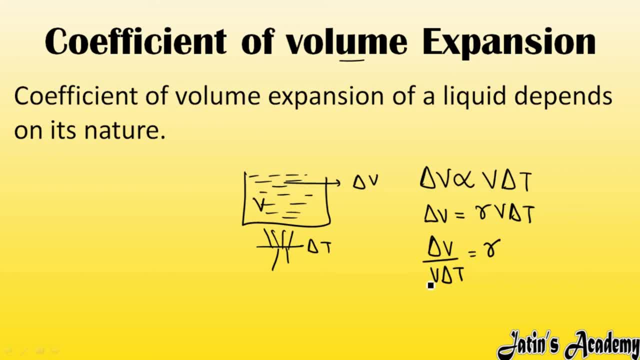 expansion means change in volume per degree, original volume per degree rise in temperature means coefficient of the volume. expansion is change in volume per unit, original volume per degree rise in temperature. and similarly we are having its SI unit also. its SI unit is per Kelvin, or you can say per degree Celsius, other unit, okay. so now we are having thermal expansion in gases. 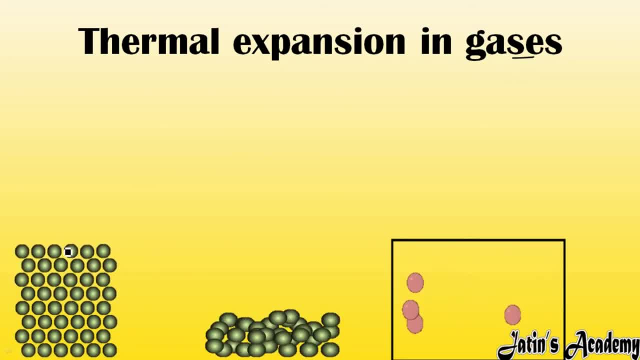 as we know, solids are having very tightly packed arrangement of the molecules, so there is a least expansion in the solids as compared to liquids. liquids are having this much space that they are expanding properly, but gaseous are having very much spaces or very least force of attraction. 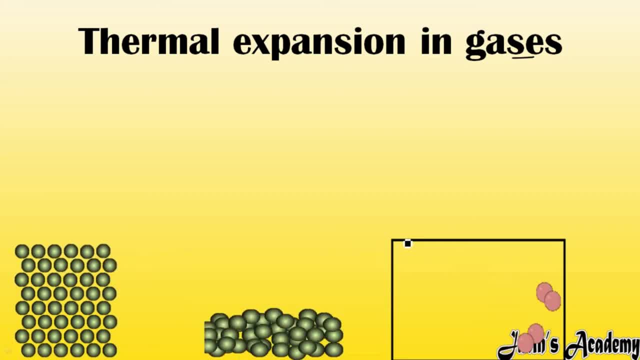 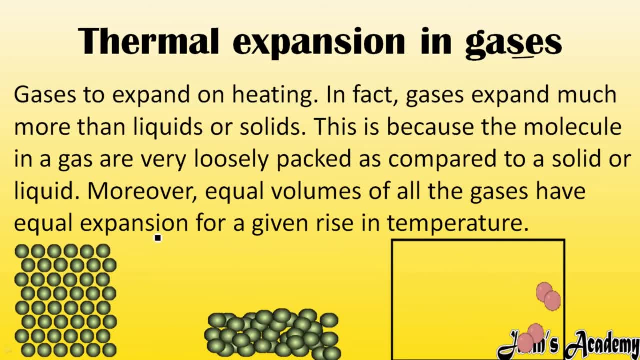 between the particles. so they are showing the very much thermal expansion. instead of solid and liquid we are having the very vast or large expansion. thermal expansion is there in the gaseous state. so by giving the same temperature to all states of matter, gaseous will show more expansion as compared to solids. 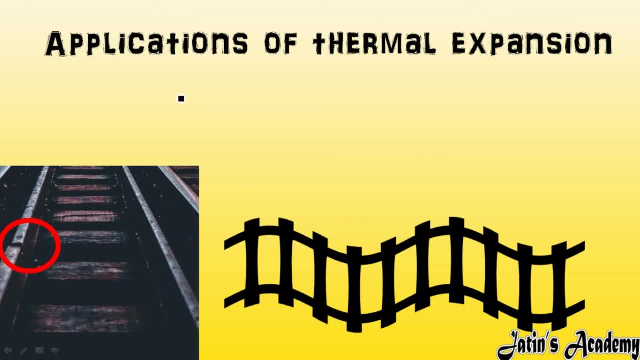 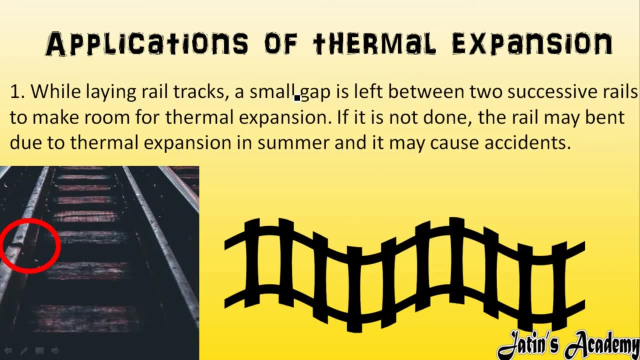 and liquids. so now we are going to see applications of thermal expansion means in our daily life, where we are going to see the thermal expansion. so very first application we are having: while laying rail tracks, a small gap is left between two successive rails. why there is a small gap between the two. 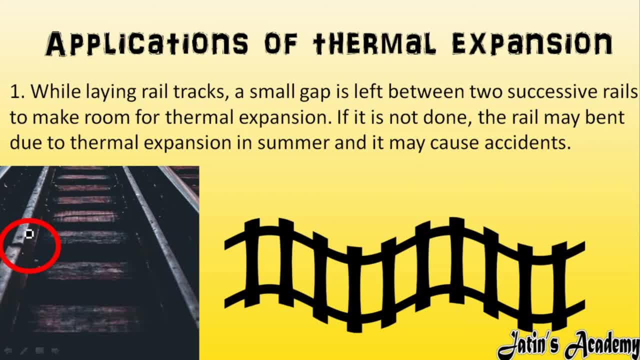 successive rails because during summer there is a thermal expansion in the solid and due to this thermal expansion in the solid, so that it can expand properly during summer, that is why some space is left between them, and if there is no space left between them, then there may be a cause of. 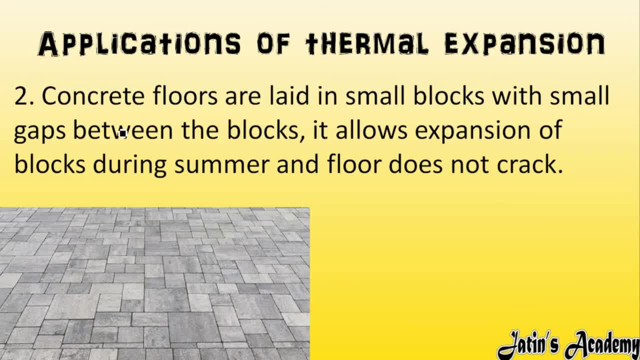 accidents due to the thermal expansion. so second application we are having concrete floors are laid in small blocks with a small gap between them, means whenever two blocks are there in the tiles, these two tiles are having some space between them. why they are having some space between them. 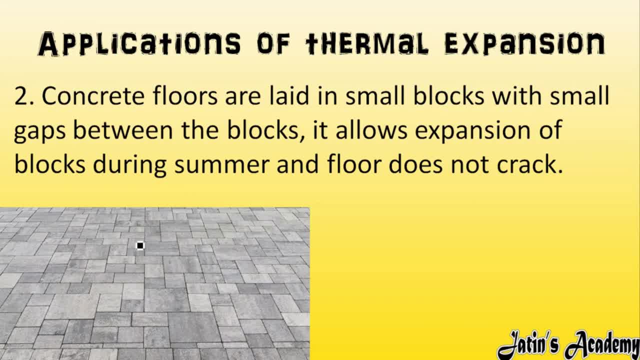 because during summer they have to expand means solid tiles have to expand so that it can take the space while expansion. that is why there is space left between the two tiles, okay. but if, yes, there is no space between the two tiles, then tiles are going to crack like this. that is why always, 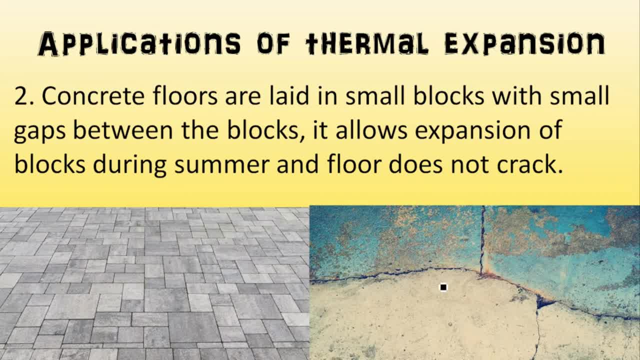 whenever there is a lid or there is a formation of the tiles on the floor, there is always some spaces left between the tiles so that in summer they can easily take up that space and there is not the crack in the tiles. next application of thermal expansion we are having when we are having 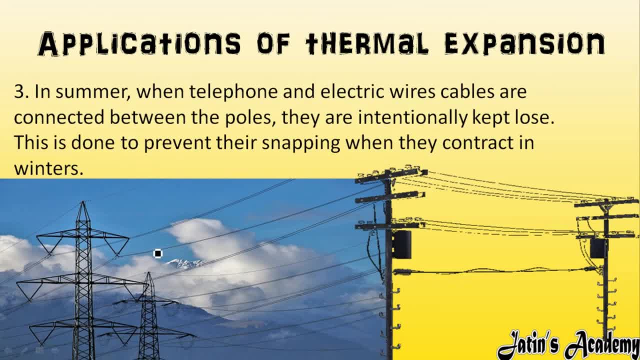 in summers the telephone and electric cables are connected between the two poles are intentionally kept loose whenever between the two poles. these wires are kept intentionally loose. why? because, as we know, during summer there is a expansion and similarly in winters also there is a contraction of the solid liquid or gas. due to this contraction, they are intentionally kept loose that whenever. 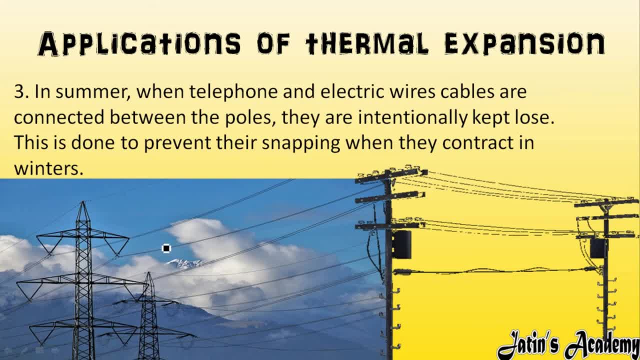 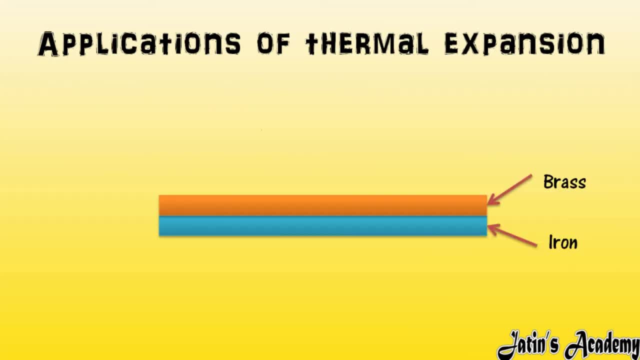 during winter they are going to contract, they will take the space and they can easily adjust itself and they can contract easily without breaking or without snagging. okay, so next application of thermal expansion we are having that we are using the biometallic strip in electric iron, electric geysers and electric ovens. why we are using biometallic strips: see 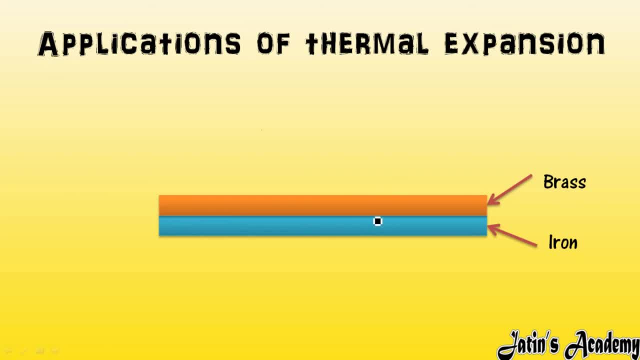 carefully. actually biometallic strip is made up of two metals. metals are brass as well as iron. for example, i'm using electric iron for the long time means whenever i'm using the electric iron it will heat up very much, obviously, but whenever i'm using for the long time the biometallic strip also is. 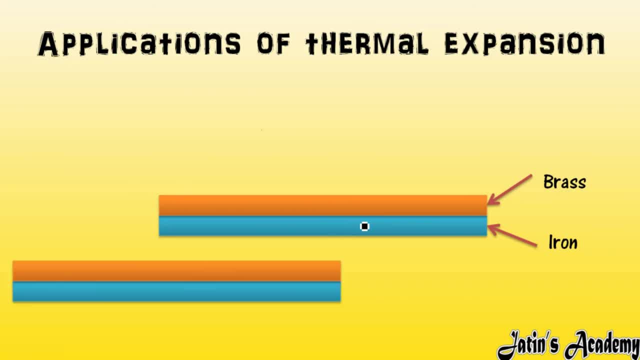 going to heaten up very much and due to this heating up biometallic strip, it will heat up. the brass expand more as compared to iron, while taking thermal expansion. there is a thermal expansion in brass as well as in the iron, so brass expand more as compared to iron whenever there is 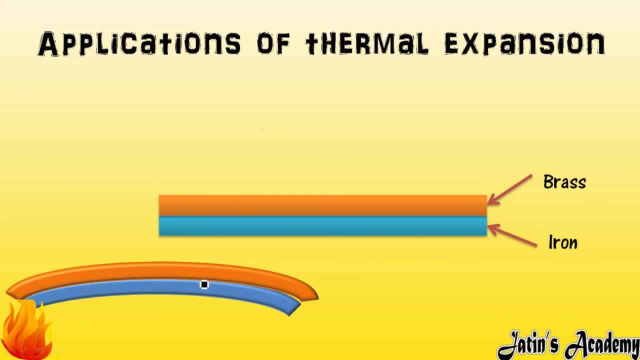 expansion of brass and iron, it will remove the contact between the electricity and the electric iron, which starts to cool down the electric iron. okay, so whenever the electric iron is going to cool it down, it will again make the biometallic strip in the straight manner. but yes, whenever 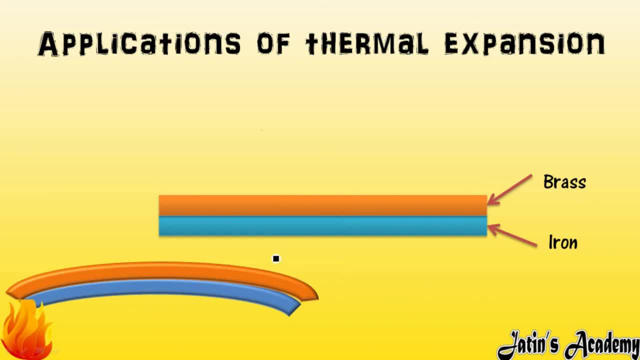 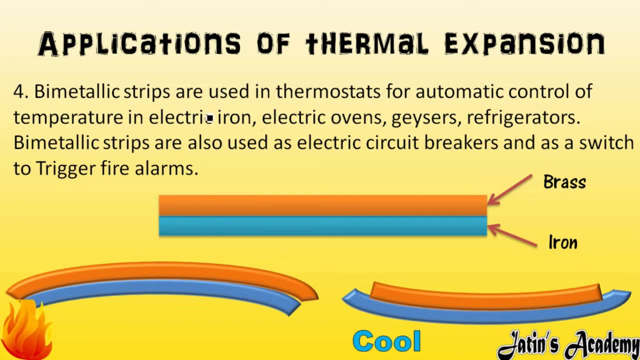 we are cooling the biometallic strip even below the room temperature. in that case, brass contracts more as compared to iron clear. so that is why biometallic strips are used in thermostats for the automatic control of temperature in electric iron electric ovens, geezers, as well as refrigerators. 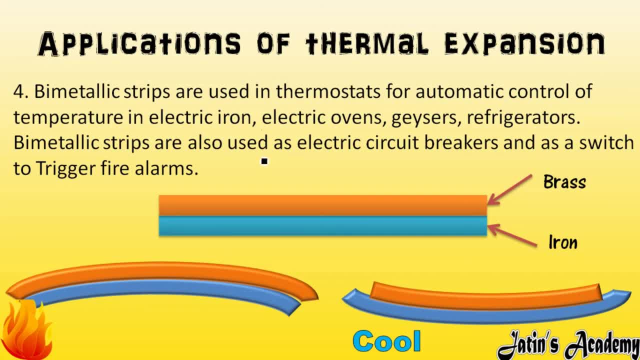 also in order to maintain the temperature in these materials. okay, even though biometallic strips are also used in mcb, that is miniature circuit breaker which is used in our main electric board so that we can just maintain the temperature flow which is coming from the main electric poles. 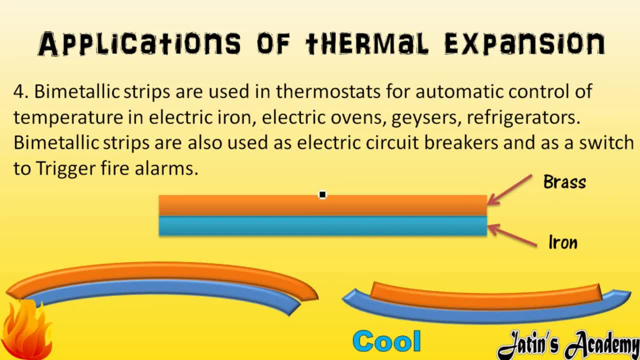 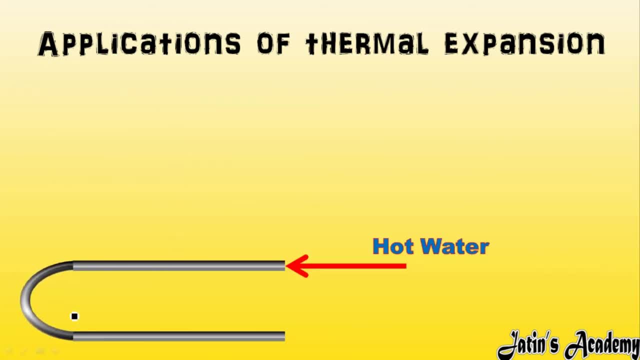 into our house in order to maintain it. we are using the mcb, and mcb also used the biometallic strip in order to maintain the temperature. so next application we are having whenever we are having any kind of metal pipes through which hot water is going to move, as the 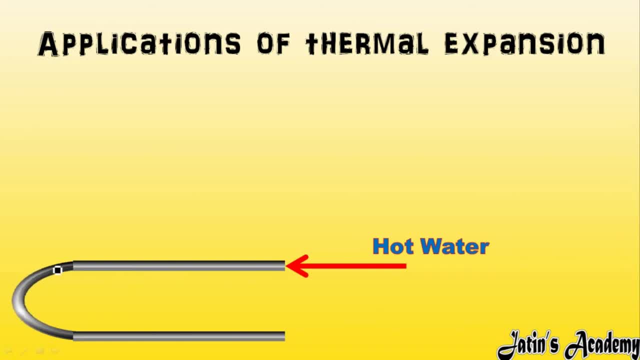 water is hot. so due to hot or due to the heat, the thermal expansion is there in the metal pipe. so always there is a space left between this metal pipe so that whenever hot liquid or any hot water is going to move from this metal pipe, it can easily adjust itself during the expansion. 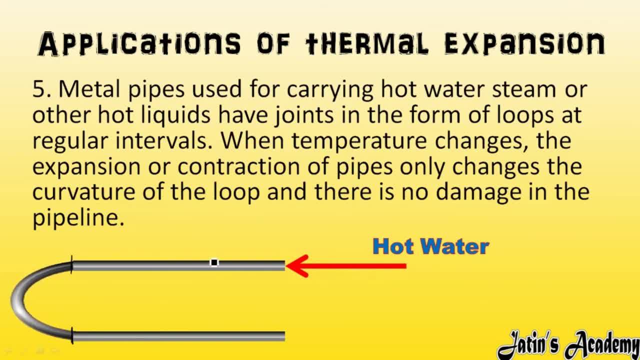 okay, so metal pipes are used for carrying hot water, steam or other hot liquids. have joint in form of loops. at regular intervals means whenever there is a change in temperature or even there is contraction or expansion in the temperature, even whenever we are putting the hot water or cold. 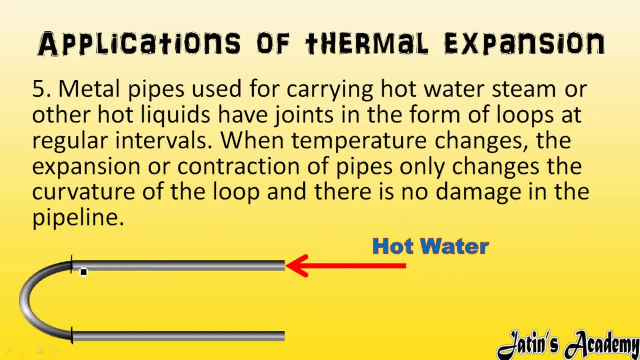 water into the metal pipe. there is a expansion or contraction in the metal pipes in order to adjust itself. in the expansion or in the contraction there is a small loops so that it can easily adjust into it. and if there is no loops at the regular intervals, then there may be a damage of the metal pipes. metal pipes may damage also. next application of: 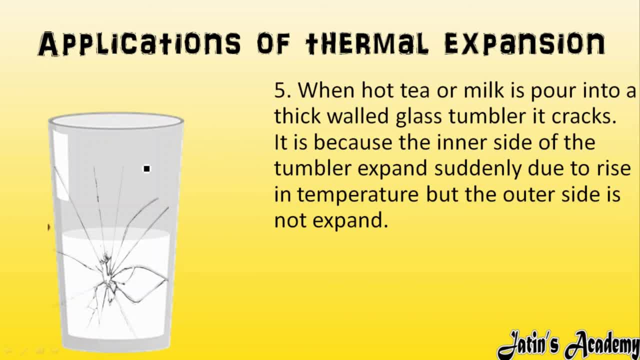 thermal expansion we are having whenever we are going to just put the hot tea or milk into the thin glass. that thin glass walls are going to break due to the hot milk or hot tea. why? because the inner side of the tumbler expand due to the rise in the temperature. means whenever we are 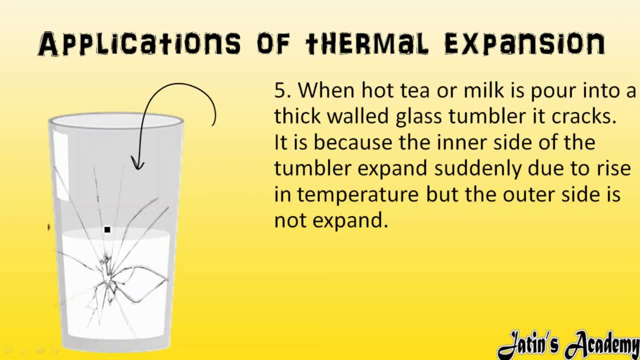 putting the hot tea into the thin glass, that thin glass is going to break. why? because from the hot thing or from the hot tea, it is going to expand from inside due to expansion, because inside there is a expansion but outside temperature is normal. due to this change in temperature, there is a 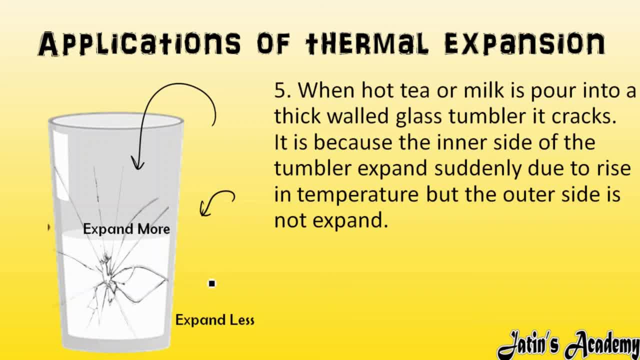 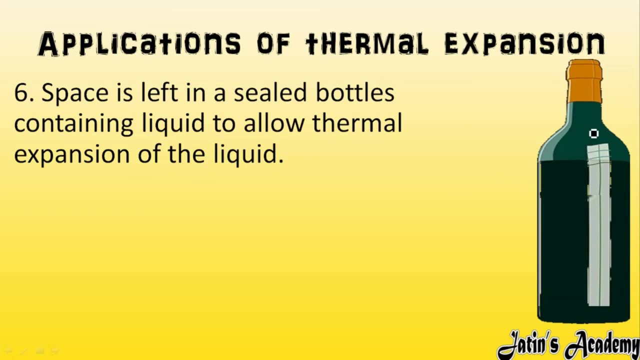 always breaking in the material. so as the surrounding expands less and inside expand more, due to this different expansion between the inside and outside, there is a breaking of the glass. so next application of thermal expansion we are having, there is always a space left between the sealed bottle. this much space is left between the sealed bottle which is containing. 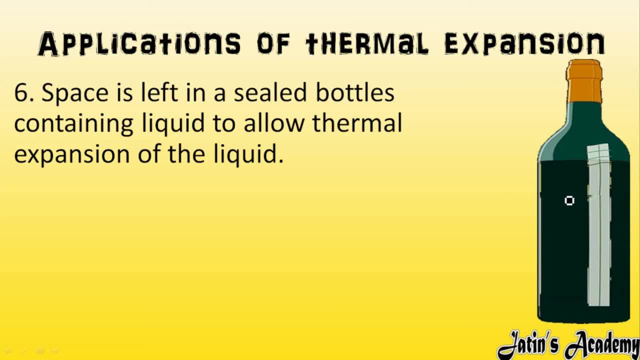 the hot tea, and the hot tea is going to expand from inside due to expansion. because inside there is a no space between the sealed bottle, then this sealed bottle may burst during the summer season, because if there is no space between the liquid molecules, then there is a no space for the 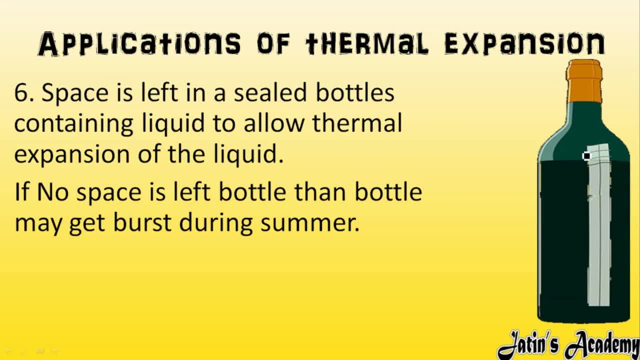 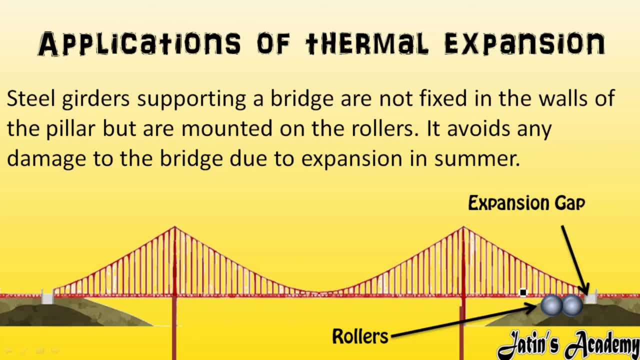 expansion also, and expansion is not there. the bottle is going to burst during the summer. so next application: we are having the steel gridders. sporting a bridge are not fixed in the walls of pillars means these bridges are not fixed to the walls of the pillars, they are just mounted on the rollers. why they are having rollers, these kind of rollers? because 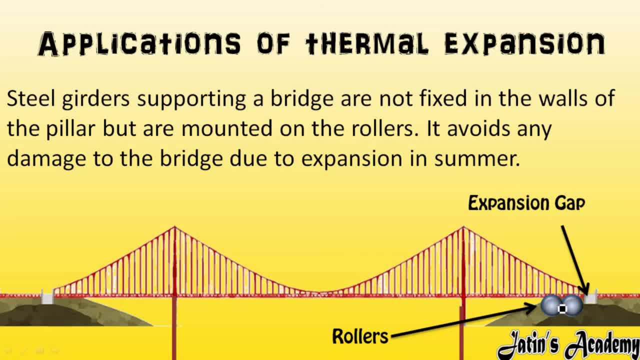 during summer. as we know, bridge is going to expand. solid is always going to expand. whenever during summer there is a expansion, it is having some expansion gap between it means whenever during summer it is going to expand, it can easily take up. the expand means the roller can easily. 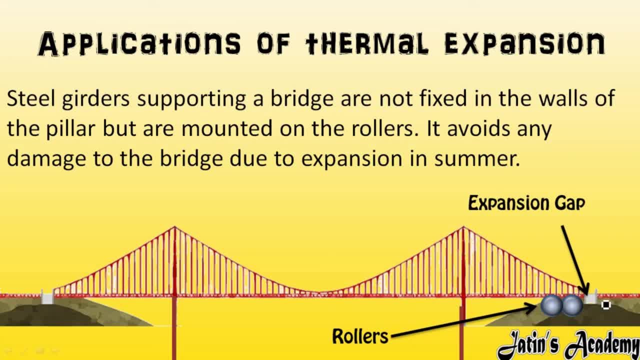 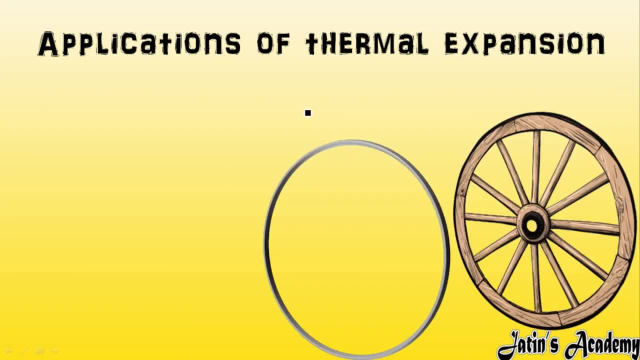 move the bridge and move to this side so that it can easily take up the space during summer. there is no damage in the steel gridder or you can say on the bridge. so next application of thermal expansion we are having in order to make the wheel of the tonga, this iron rim diameter is always less. 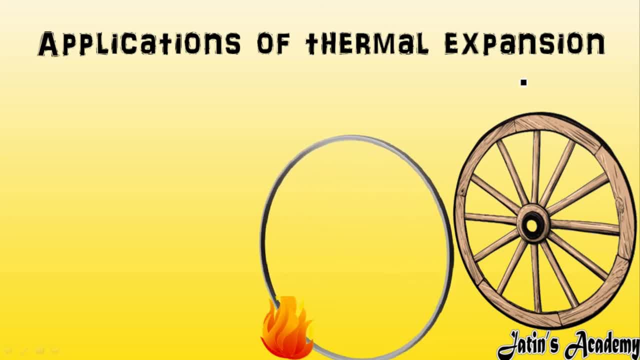 as compared to this wooden wheel diameter. why? because and whenever we are going to fit this expanded ring on the wooden wheel, it is going to adjust itself. means afterwards there is a cooling effect. means they are pouring the cold water onto it and after cooling effect there is a contraction. 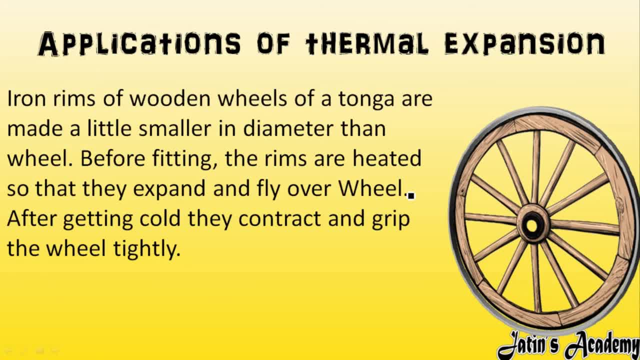 it can easily adjust to the wooden wheel. so iron rim on the wooden wheel it can easily adjust to the wooden wheel. so iron rim on the wooden wheel of the wooden wheel of the tonga are made little smaller in diameter as compared to wheel. because whenever, in order to fit the iron rim into the wooden wheel, this iron rim is firstly going to 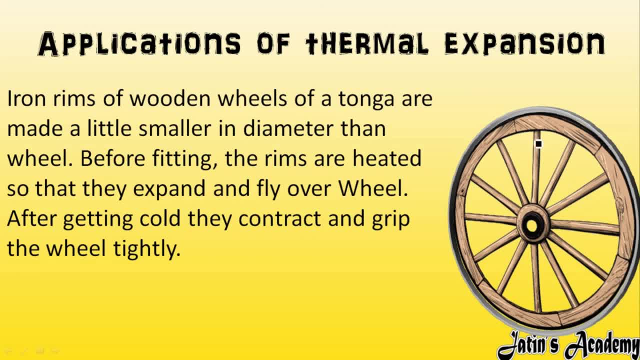 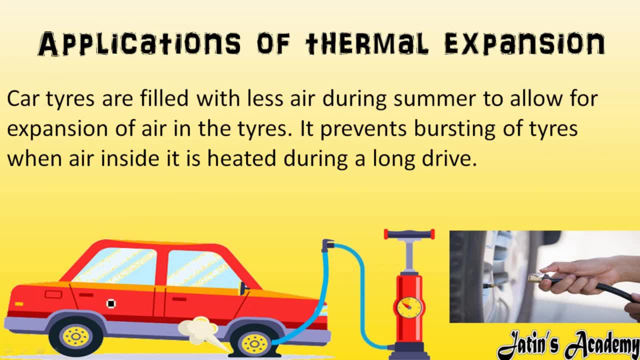 heat and up. due to heating up, there is an expansion in the ring. after getting cold, this iron rim can easily adjust itself into the wooden wheel. next application we are having: car tires are always filled with less air during summers. why? because, as we know, during summer there is a thermal 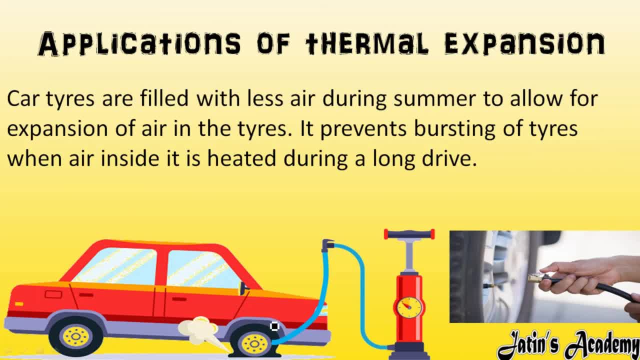 expansion in the solid liquid as well as gaseous. also why we are filling it with the less air because, as we know, during summer there is an expansion in gaseous. also, in order to prevent the tire from the bursting, we are just filling the car tires with the less air. this is 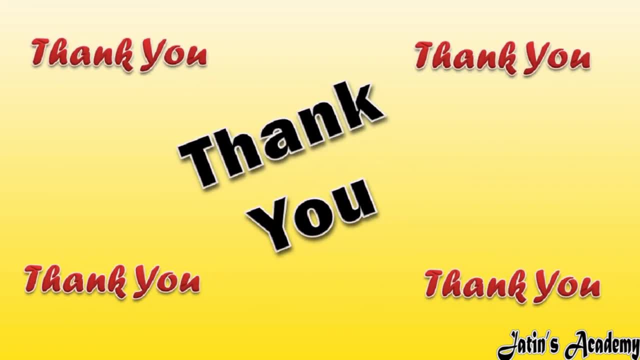 all about your chapter number six, that is, heat transfer of class eighth iclc physics. if you like the explanation, please like it, share it and subscribe our youtube channel. thank you so much.